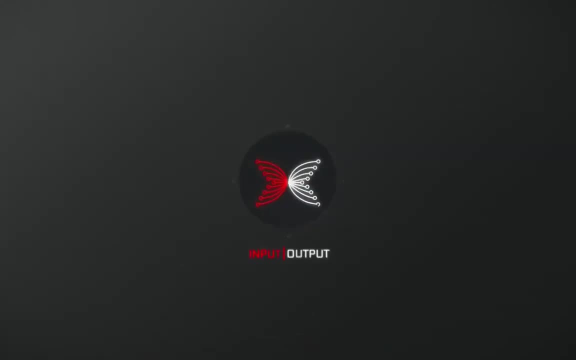 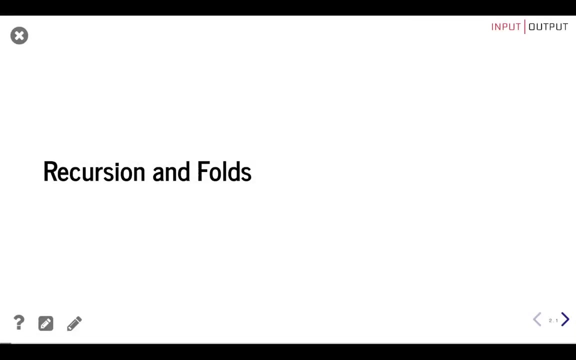 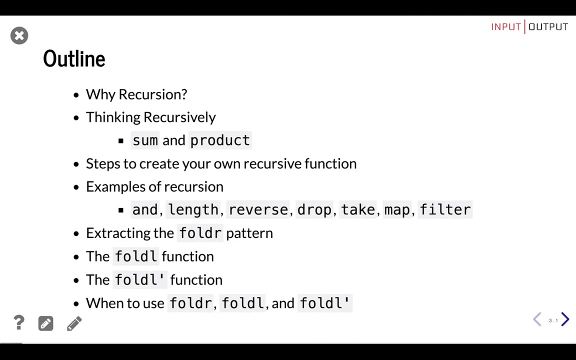 Welcome to the recursion and folds lesson. We'll start by answering: why do we need recursion? Then we'll learn how to think recursively and apply that thinking to produce the sum and product functions. Then we will go over a few steps to make it easier to create your. 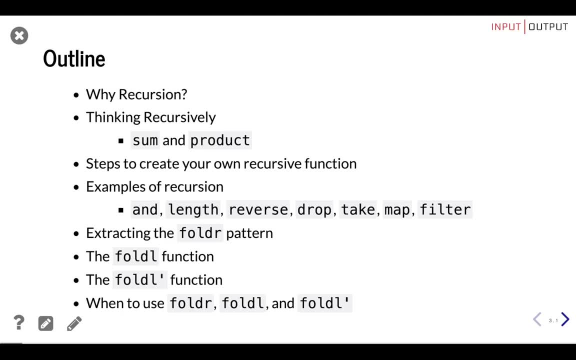 own recursive functions and apply those steps to create a bunch of functions, Then we will identify a pattern and extract it, calling it fold R pattern, And from that we'll learn about fold L, fold L, prime and when to use each one. Let's get started. Why recursion? 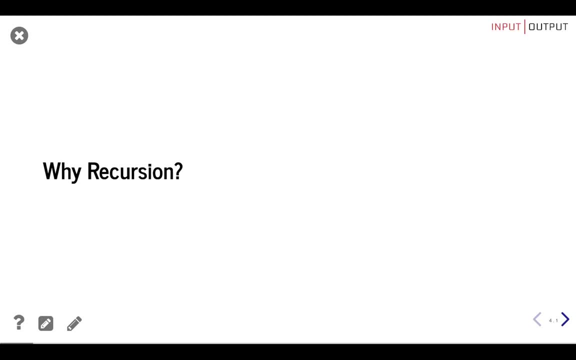 One of the most basic functionalities necessary in any programming language is repetition. For example, you have a list of objects and you want to do something to all of them, one by one, Or you want to do some calculations five times with different values. In imperative programming languages, these repetitive tasks are dealt with using iterative. 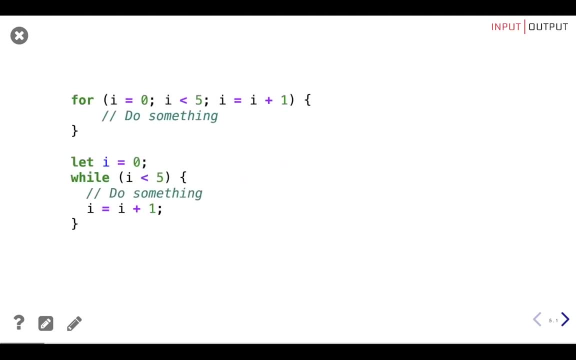 loops. For example, in JavaScript you can have something like this: a for loop and a while loop. In the for loop, you instantiate the I variable with its first value. You also specify the limit up until when the for loop should run and how to mutate the variable. And in the while loop, you first instantiate the 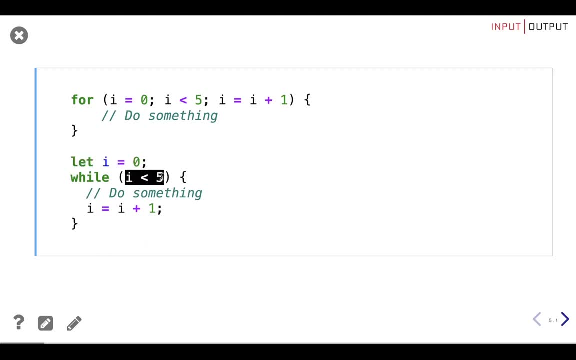 variable, set for how long it will run and mutate the variable. If we try to create something like this in Haskell, we will have a big problem, And that's the I variable. As we covered in lesson one, Haskell is a purely 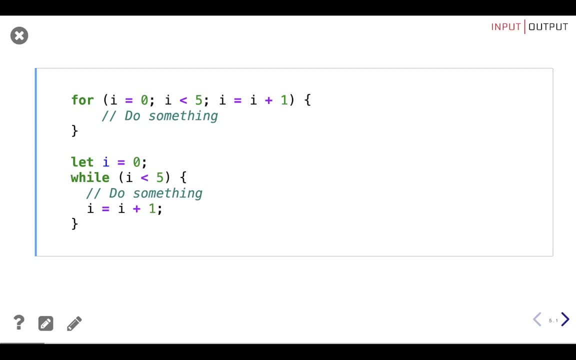 functional language. But these two code blocks rely on changing I on each iteration. That means they have the side effect of updating a global state as the program progresses. So in Haskell we do not have this built-in looping function. Instead we have recursion. 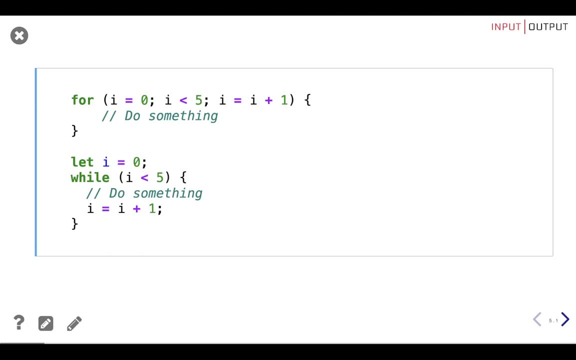 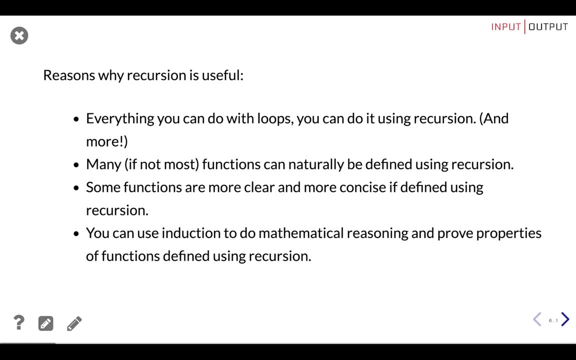 And how is recursion better than looping? you say. Here are a few reasons. Everything you can do with loops, you can do it using recursion. And on top of that there are even programs that you can recursively define that cannot be written using for loops. Many, if not most, functions can naturally be defined using recursion. 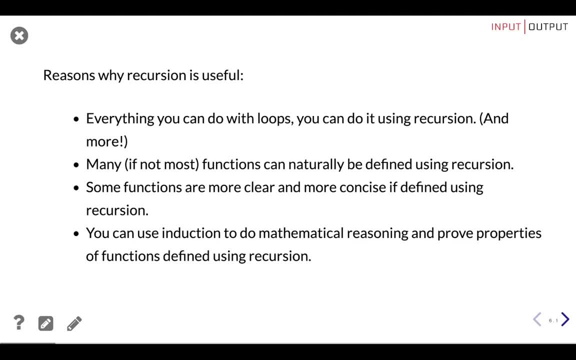 This answer is for me. This means that the way you abstractly think about the function and the way you write it using recursion is highly similar. Also, some functions are more clear and more concise if defined using recursion. And finally, another one is that you can use induction to do mathematical reasoning and 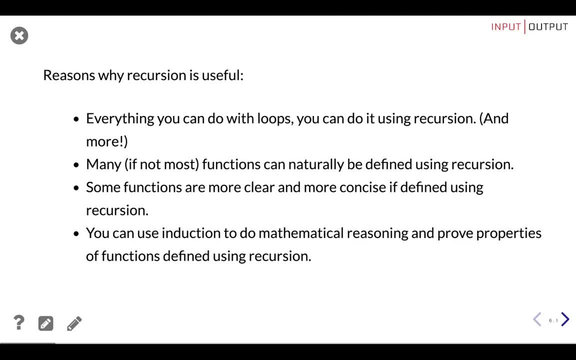 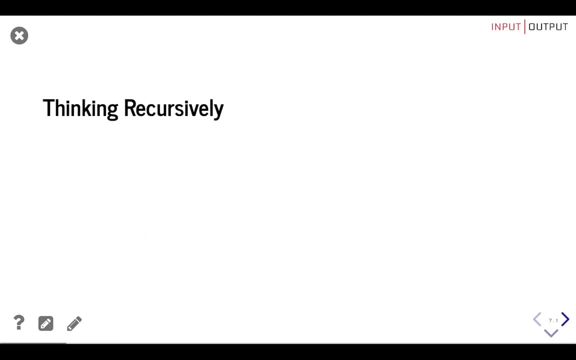 prove properties of functions defined using recursion. This is more advanced, but incredibly powerful. Okay, so now that you know that you're about to learn a pretty powerful concept, let's dive in. Recursion occurs when a thing is defined in terms of itself. 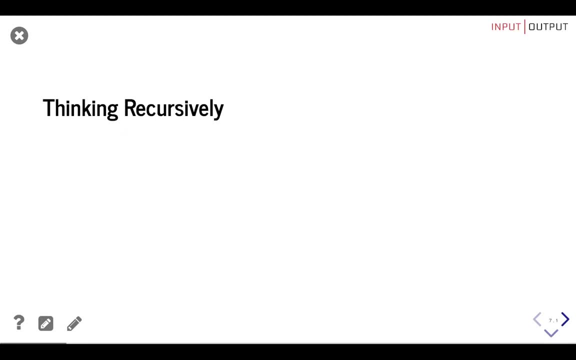 So a recursive function is one that is defined in terms of itself. That's it. The concept is really simple, The implementation is simple. The implementation is simple. The implementation is what gives most of the trouble. So we're going to start by defining a function using both a for loop in Python and a recursion. 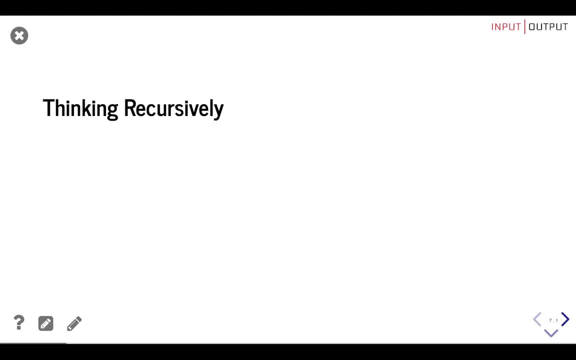 in Haskell to highlight the difference in the way of thinking about the problem. For example, let's say that we want to calculate the sum of a list of numbers. Both Python and Haskell have the sum function that already does that, But this time we're going to create it from scratch. 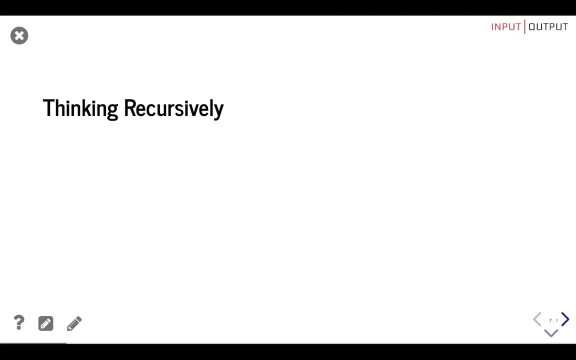 So you can do it in a couple of ways. In imperative languages you will write something like this: Here you are describing step by step what the program should do. We create a function named sum that takes a list. Then we create the variable called total, with an initial value of zero. 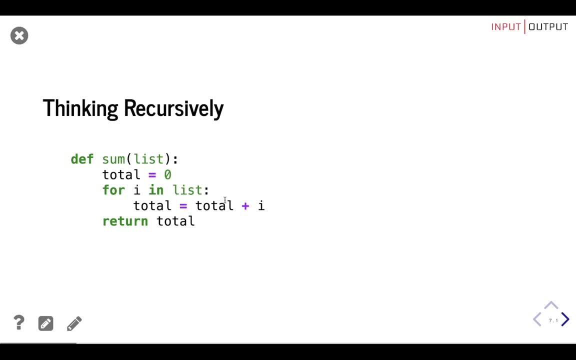 Then, for each element on the list, we take total, add the value of the element and overwrite the value of the element. Okay, so we're going to write this function as before, So call it a list of total, using the assignment operator. this is not equal. this is an assignment operator, so we 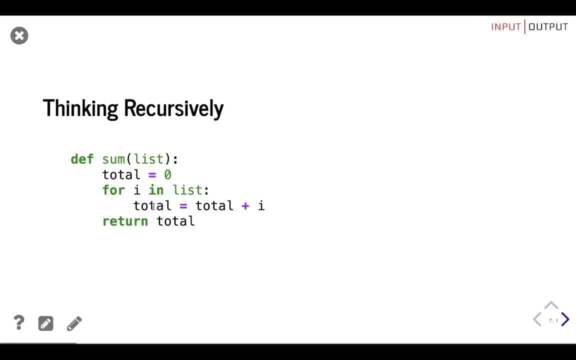 are overriding the value of total, we are mutating total and, after the loop finishes, the function returns the total value. as you can see, in imperative languages we use a sequence of statements to determine how to reach a goal, in this case, the sum of the elements in the list. 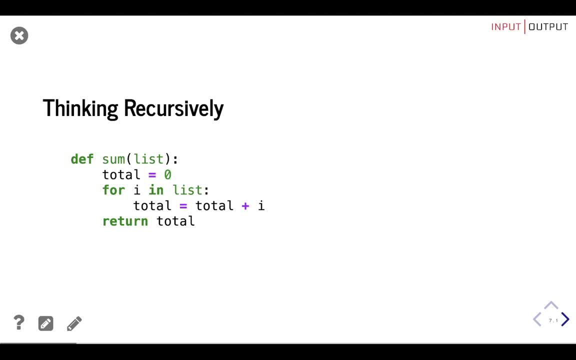 to easily write recursive functions. you have to get rid of that way of thinking and embrace declarative programming, where you declare what things are instead of how to obtain them step by step. now let's define the same function, but in haskell. as always, the first thing we need to do 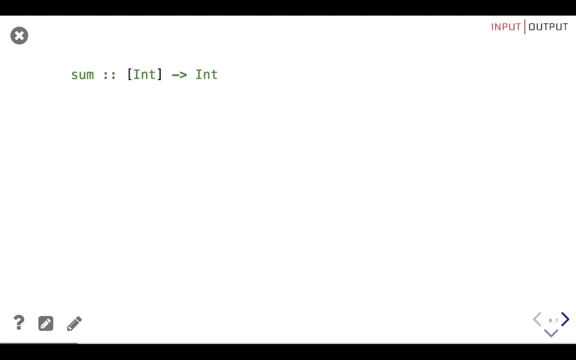 is to write the type signature. so we know it takes a list of numbers. we choose them to be integer and we write the type signature. and we write the type signature and we write the type integer and returns an integer. now, based on what that function is, one that takes a list of numbers. 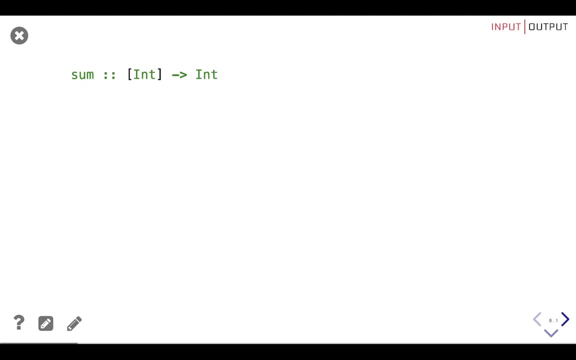 and returns its sum. the next is to look for edge cases. we take a list as an input. what happens if the list is empty, for example? well, in that case we know that the sum of an empty list is zero. we can start by defining just that now. besides that, there's the case when there are elements inside the list, so we can also add that. 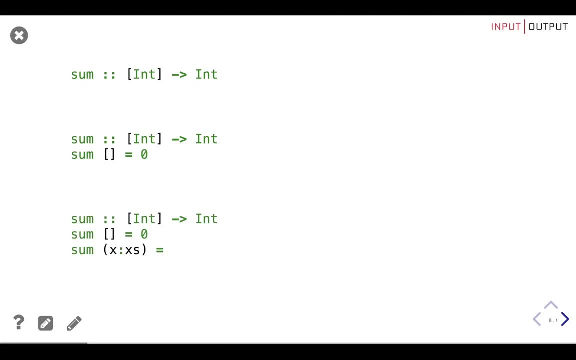 case if we think about what the function sum is. on the second definition, it is a function that takes a non-empty list of things and adds them up, which is the same as adding x, the first value of the list, to the result of adding all the ends in the x-axis. 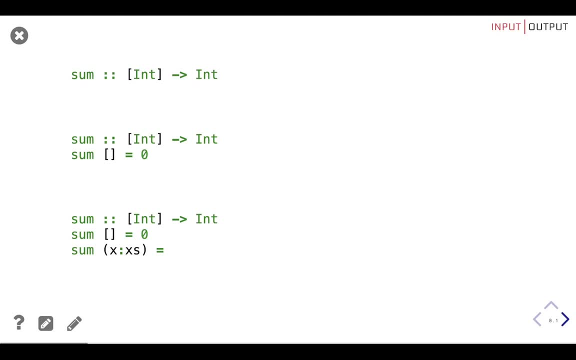 the rest of the values. so we could do something like this: and now we need to find the sum of all the elements in xs. but wait a minute, we already have a function to do just that. it's the same that we are defining right now, so we can just use it and apply it to the rest. 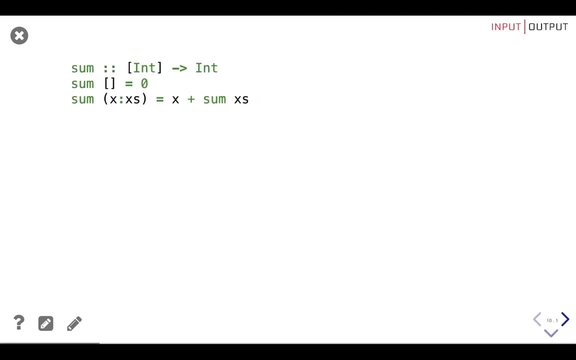 of the values. and there you go. we implemented our first recursive function. why? because we defined some using itself. let's see what happens if we use the function. for example, let's calculate the sum of a list that contains all the integers from zero to five. let's see, step by step, when we 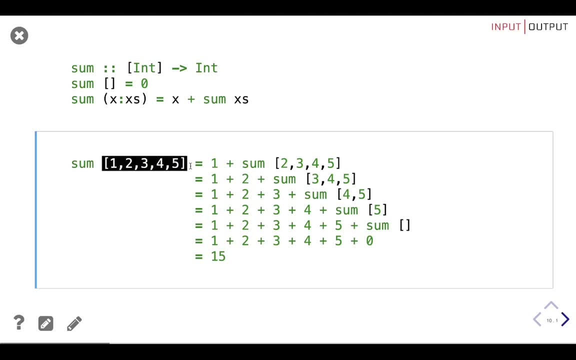 use the function, we first provide a non-empty list, so we fall. in this case we take the first value one, we add it to the recursive or sum to the rest of the values, So it's one plus sum of a list that doesn't contain one anymore. 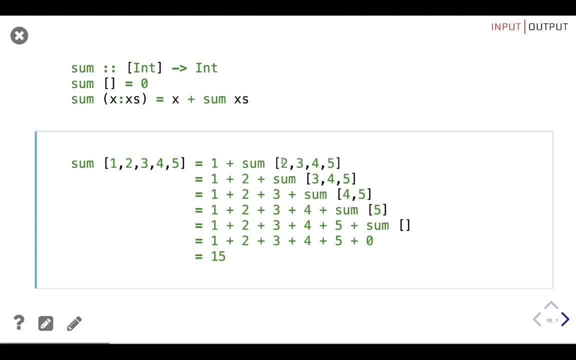 And because this is a known empty list, we do the same: Take the first value and add it to the recursive call of the rest of the list And we keep going until we hit the base case or the edge case. When sum is applied to an empty list, we return zero. 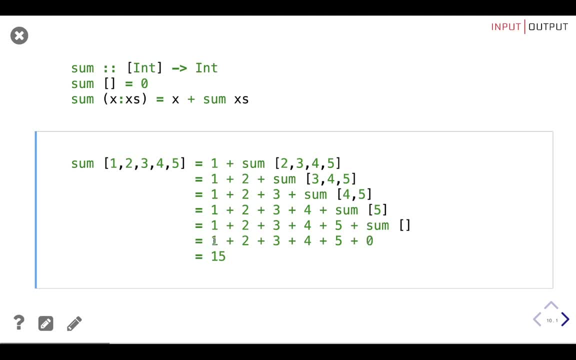 So that's what we have here, And finally, we have an expression that we can easily reduce to 15.. And that's how Haskell evaluates our function. Notice that the base case is the one that allows us to stop the recursion and have a result. 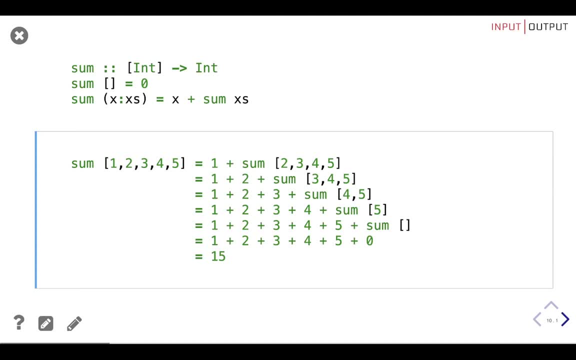 If we define the recursive function without a base or an edge case, it will crash or run forever. So in a few words: with loops you change the context with a mutating accumulator that wraps the steps to determine how to reach the goal. With recursion, you wrap the function with itself. 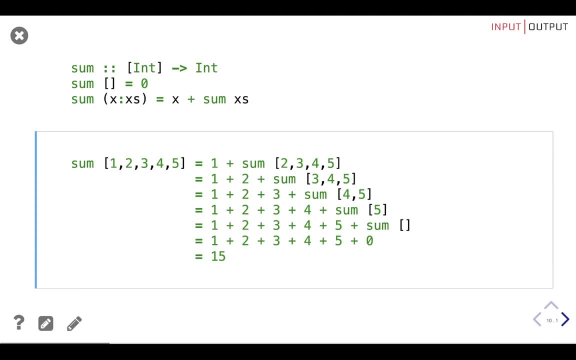 which creates a new context with the desired mutation, In this case a changed list, And that function in turns calls itself again, set it up, its own new context, and so on and so forth. Now, even though this was a complete walkthrough on how to create this sum recursive function, 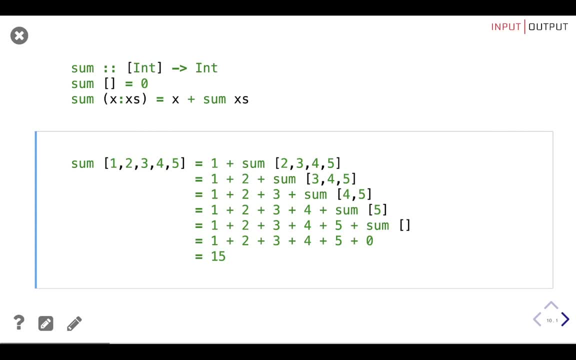 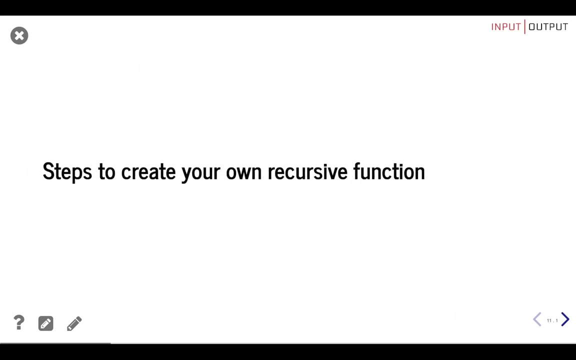 the reasoning. maybe it'll be too specific to apply to other functions. To make it easy for you to create your own recursive functions, we will write a generic step-by-step that you can apply. to any case, Let's dive in. I prepared a slightly modified version of the steps created. 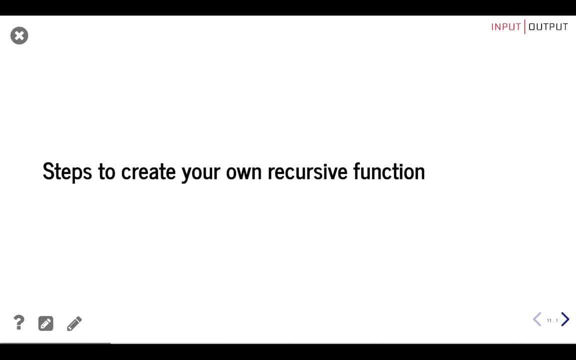 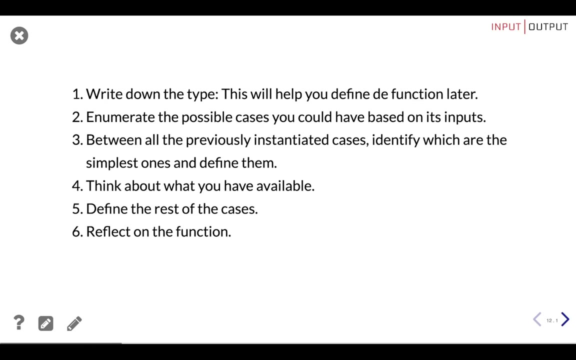 by the one and only Dr Graham Hutton, Renowned researcher, teacher and board member of the Haskell Foundation. So you know these are the real deal. First, as always, write down the type. This will help you define the function later. 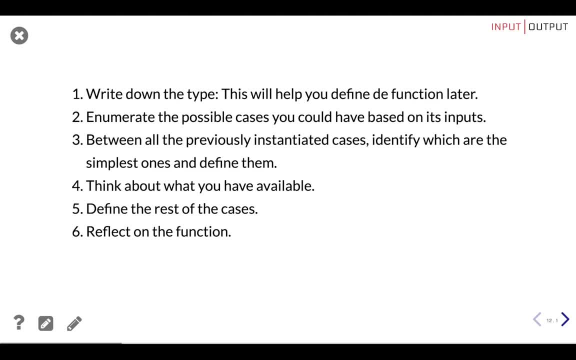 and you should always define the type first, anyway, even if you're not defining a recursive function. Second, enumerate the possible cases you could have based on its input. Start with the start standard ones that we will cover in this lesson, and change or refine them as needed. 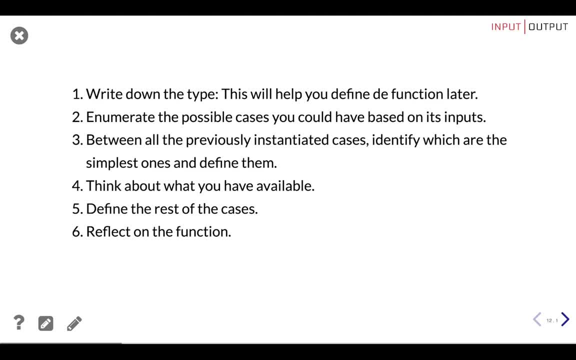 Third, between all the previously instantiated cases, identify which are the simplest ones and define them. These often are the base or edge cases. Or think about what you have available to you: Parameters, functions, operators of that specific type, et cetera. 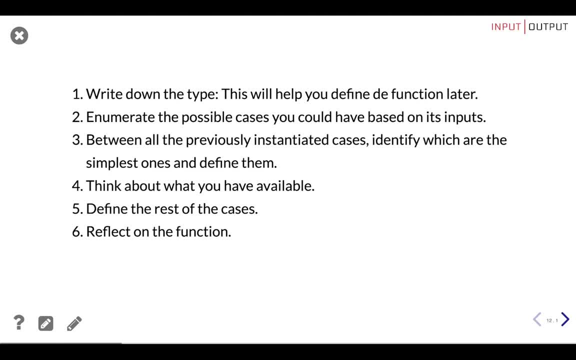 Use those to define the rest of the cases And finally reflect on the function. Can the definition be simplified? Can the signature be generalized? Does it do what you intended to do? You don't always have to go through these steps. Once you feel comfortable, you can skip a few. 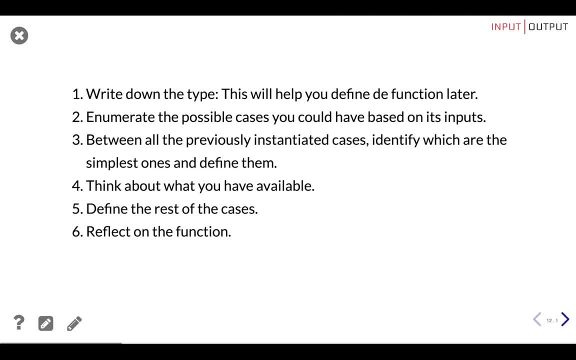 or even write the function right off the bat. In general, the base or edge case is usually the base case. In general, the base or edge case is usually the base case. In general, the base or edge case is usually the base case. 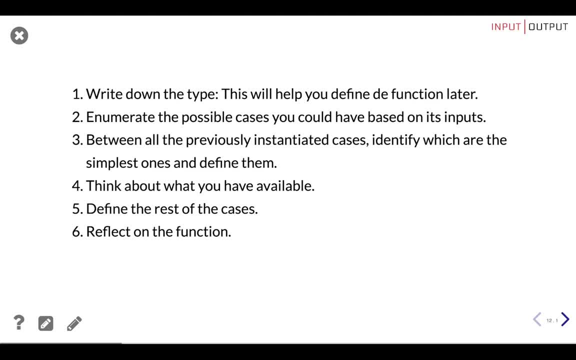 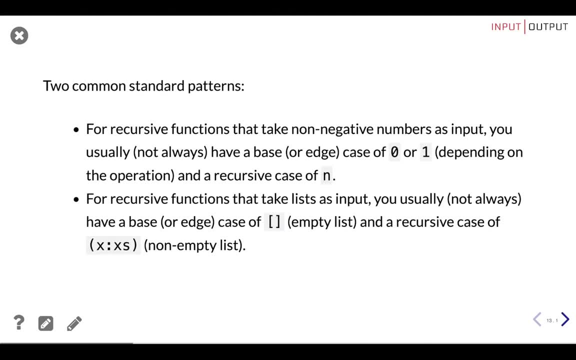 The identity case, A case that doesn't modify the results but just stops the recursion. Here we have a few examples. Here we have a few examples. These are two common standard patterns For recursive functions that take non-negative numbers as input. you usually have a base case of zero or one. 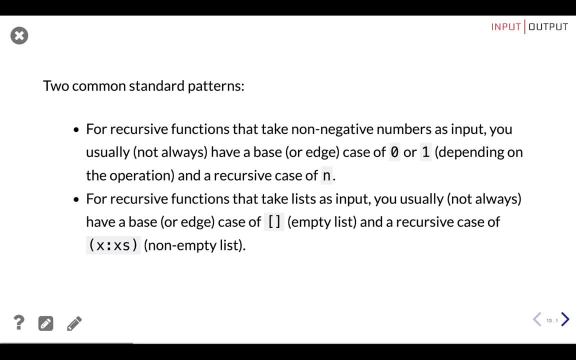 Depending on the operation and a recursive case of n, any other number that is not zero or one. Why zero or one? because those are the identities of many of the operations you will use. For example, zero is the identity operator for plus. 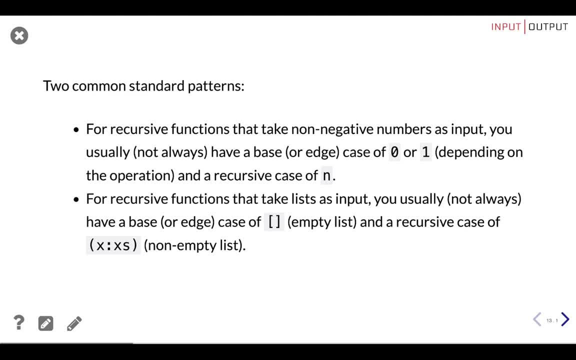 because if you add zero to something, it's still that something unchanged, One for the product, operator, and so on and so forth. Another case is for recursive function that takes lists as input. In this case, you usually have a base case of the empty list. 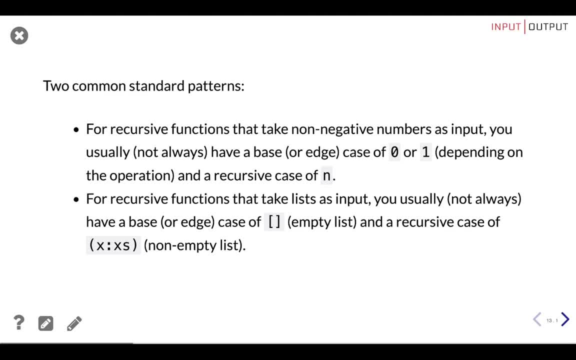 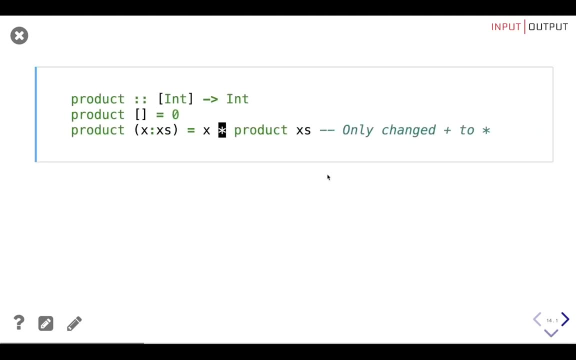 and the recursive case of the non-empty list. So, taking that into account, if we want to modify the sum function to calculate the product of the elements and we just change the recursive case like this, we just change plus for the multiplication operator. 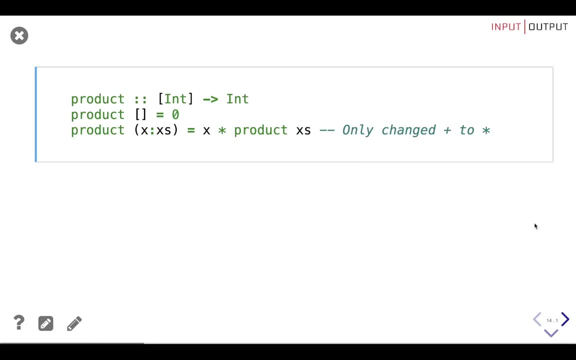 we will run into the problem that the function will always return zero because all the elements of the list get multiplied by zero at the end of the recursion due to the base case. So instead, the correct way to define the base case for product is to provide the identity. 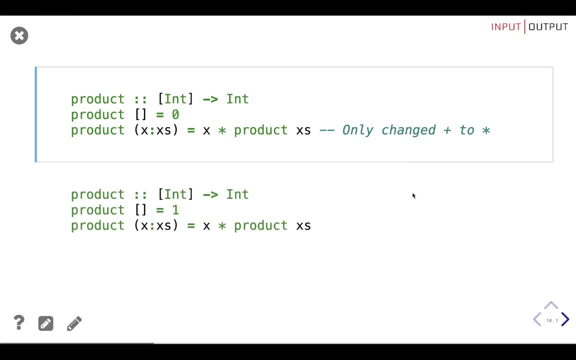 for the product operation, which is one. And there you go, We have our second recursive function defined. Practice is what gives you the intuition needed to quickly define recursive functions. So let's define a bunch of functions to get that intuition going. Let's start with the and function. 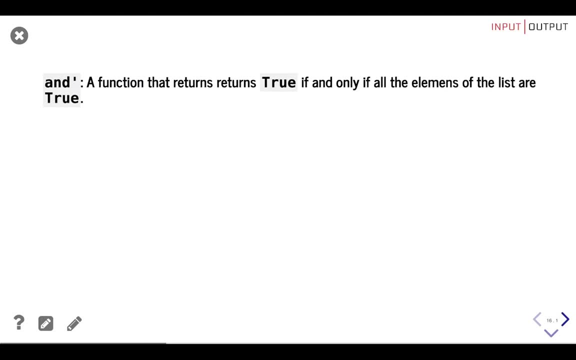 a function that returns true if, and only if, all the elements of the lists are true. I added the prime to the names of all the functions that we're going to define because they all already exist in Haskell. After this lesson, you won't need to actually define them in your code. 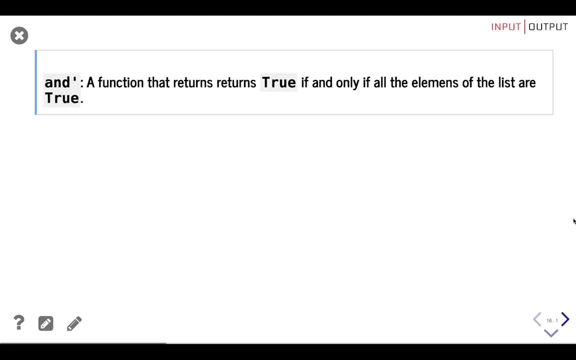 You can just use them. The and function takes a list of booleans. a returns a boolean. translating that to the type is just this: a list of booleans to a boolean. Now, because it takes a list, we will define the standard case for lists. 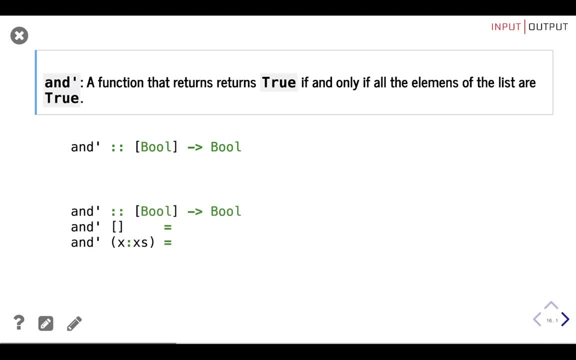 the empty list and the non-empty list. The base case might be not that obvious. Sure, we have just two values to pick from, because it's a boolean, but which one? We will start with the recursive case. Now let's think about. 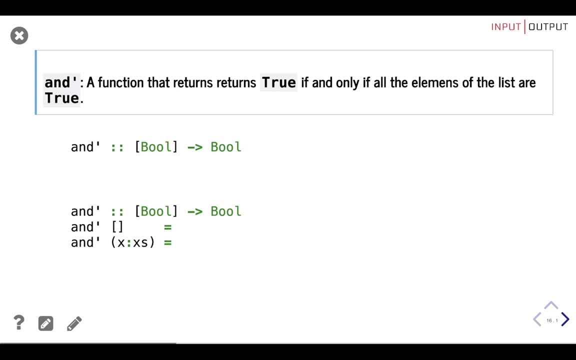 what we have available to us, Because we're dealing with a boolean. we have access to all the boolean operations And there's one that does exactly what we need, but just for two values, and that's the and operator. The and operator takes two values. 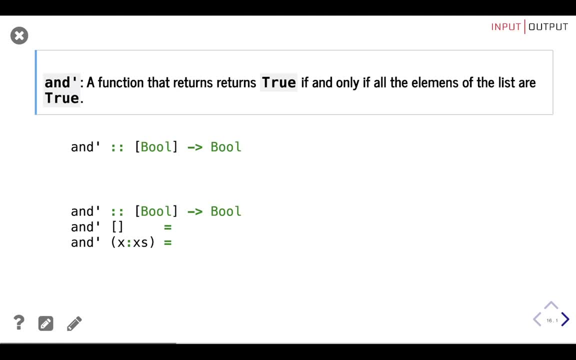 and if both are true, it returns true. Any other case it returns false. So the first element there, which is the element combined using the and operator with the result of processing the rest of the list, gives us the reci result. 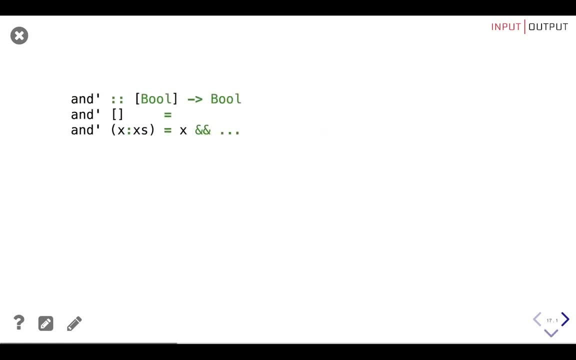 So we can do just like this, to combine the first value with the result of processing the rest of the list. And now we have to return true if, and only if, all the elements inside of X, S are true, Meaning that we need the same function. 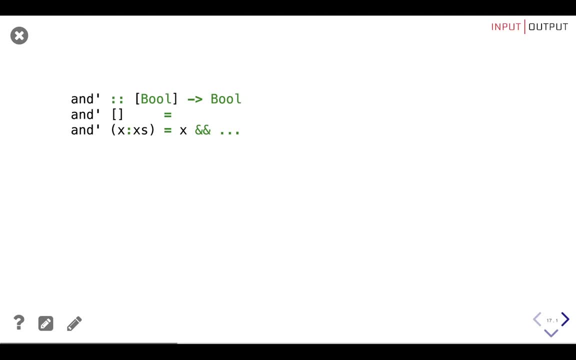 we are defining right now so we can use it and apply just to XS. And now the base case is obvious. If we use false, it doesn't matter which list we process, we will always return false because the AND operator having false to its right. 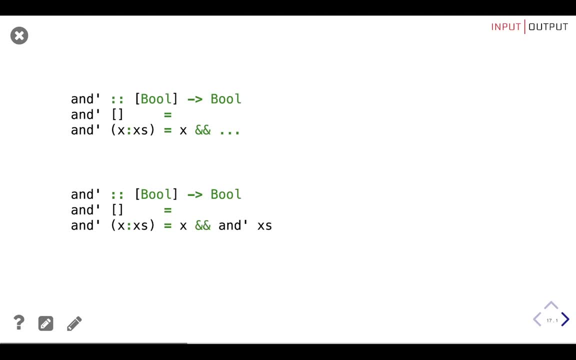 it will always equals false. But if we use true, we won't modify the result, because the result of applying AND true to its right depends on the missing left side. So if there is a single element that isn't true in the list, it will give us false all the way into the end. 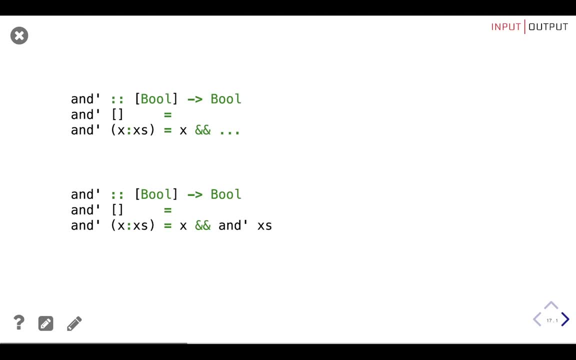 else it will give us true. Another way to figuring this out is to figure out that true is the identity for the AND operator Replacing the base case. we get the final result And, as you can see, if we have a single false. 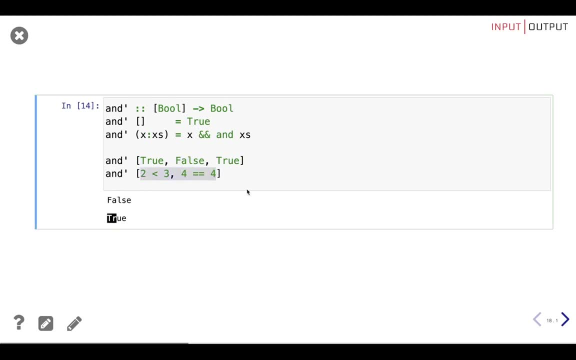 we get false. but if we have all trues, we get true. So it works as expected. In this definition, there's not much we can do about simplification, so let's move on. Now we're going to define the length function. 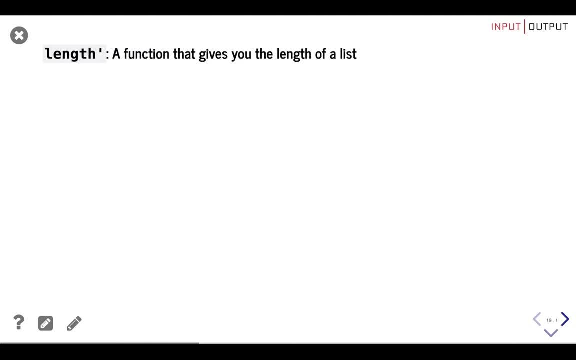 a function that gives you the length of a list. To calculate the length of a list, we have to take a list and return an integer, And because, in principle, we won't operate on the elements of the list, we can use polymorphic type for the list. 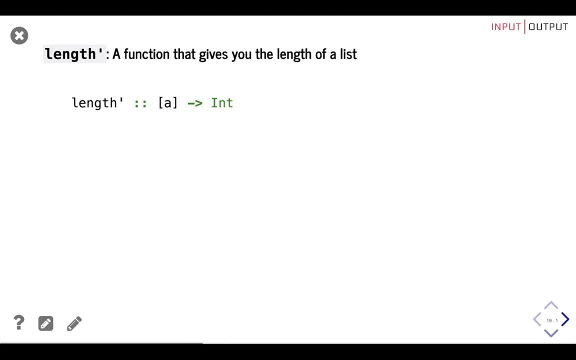 Because it takes a list. we will define the standard cases for lists. Looking for easy cases, we can identify that the length of an empty list is of course zero, so we'll replace that. And now for the recursive case. We can calculate the length of a list using the list function. 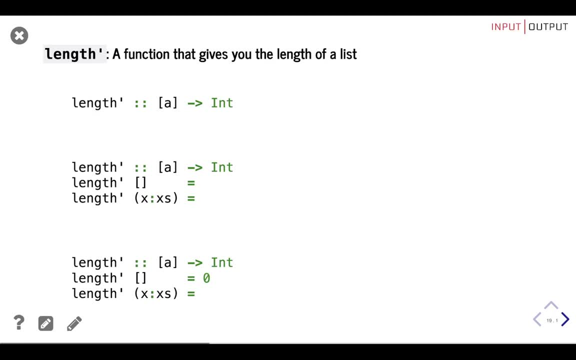 the length of a list if we add 1 for each element of the list right, And because we have the first element, x, singled out by pattern matching, we can add 1 for it and recursively calculate the length of the rest of the list like this: 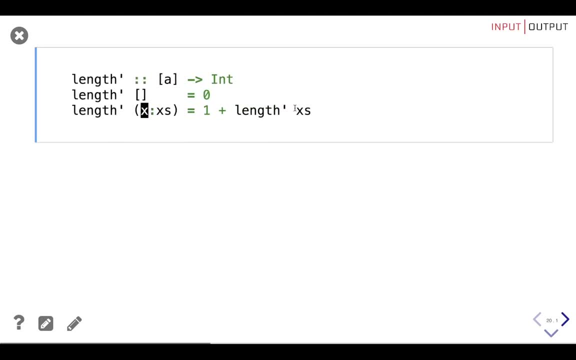 As you can see, because we are not passing down x, this list will be shorter and shorter until it's empty when we add 0. So we will get a bunch of 1s adding together until we get a 0, and that's the length of the list. 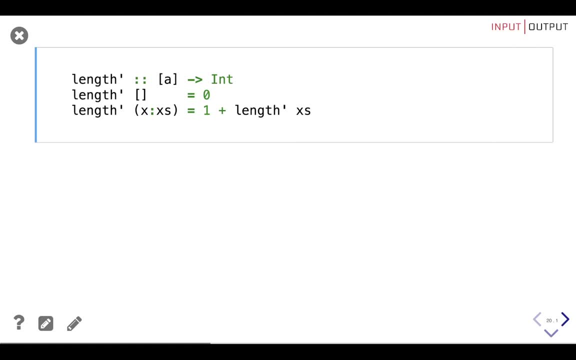 That 1 could be our final function. But, looking for improvements, we actually see that we don't use x in the body of the recursive functions, So we can ignore it in our pattern matching to obtain our final function. So far, so good. 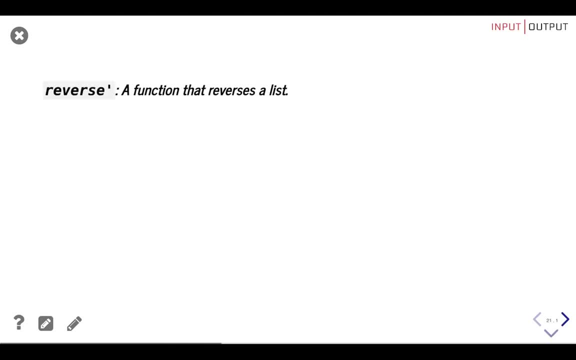 Now let's implement the reverse function, a function that reverses a list. To reverse a list, we have to take a list of elements and return a list of elements, And because in principle again, we won't operate on the elements of the list, 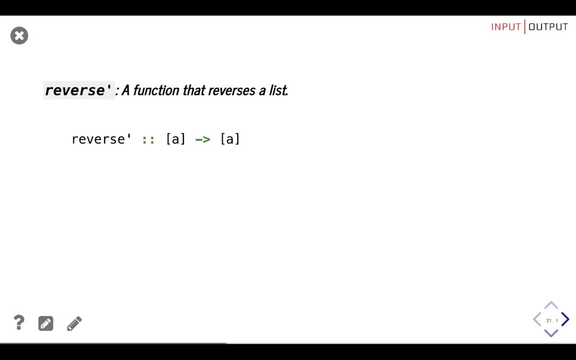 we can use a polymorphic type like this Because it takes a list. we will define the standard cases for the list. We see that the reverse of the empty list is just the empty list. so that's it. That's the easy one and that's also the base case. 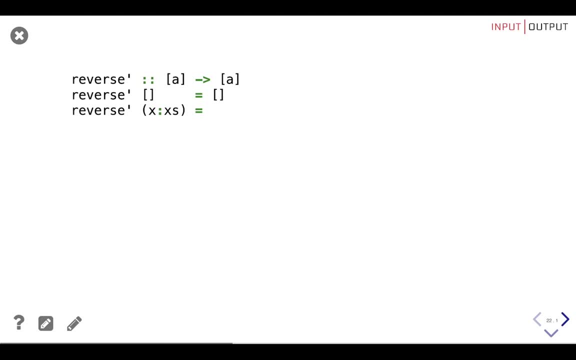 because it's not recursive. If we take the first element, because it's already singled out by pattern matching, and put it at the end, and we keep doing that until we reach the end of the initial list, we will obtain a reverse list. 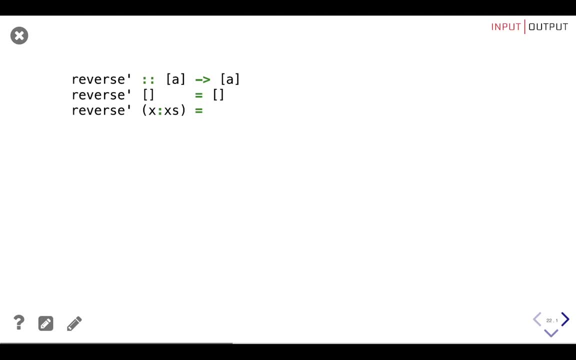 So we just need to take x, put it at the end and do the same recursively until we run out of elements, which is our base case For this. we can use the concatenator operator and recursively call to the left the reverse with the rest. 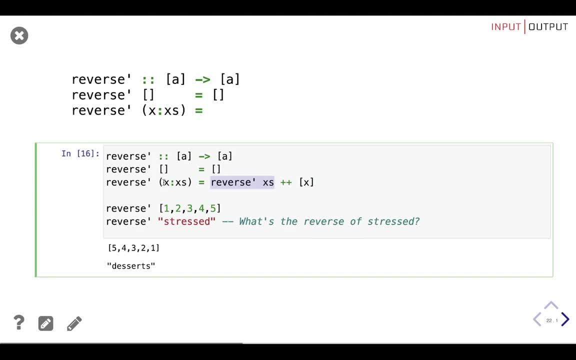 of the list and to the right, because previously it was to the left of x's. now we need it to the right- is a list containing just the single element we want to move from the front to the back. We can use this function with any type of list. 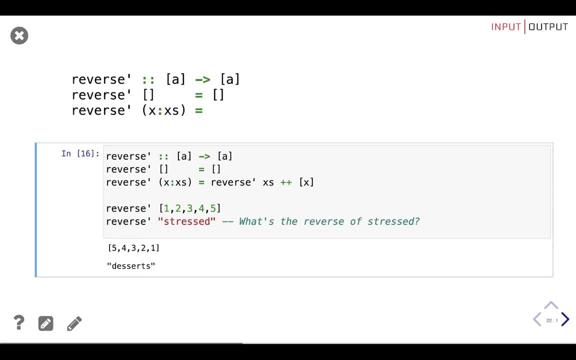 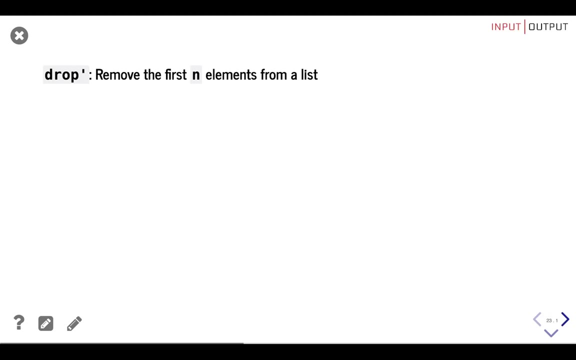 and we get the result that we wanted. Okay, we saw enough easy examples. Now let's do something a little bit more complicated. We will define the drop function. Drop function removes the first n elements from a list. It takes an integer and a list and returns a list. 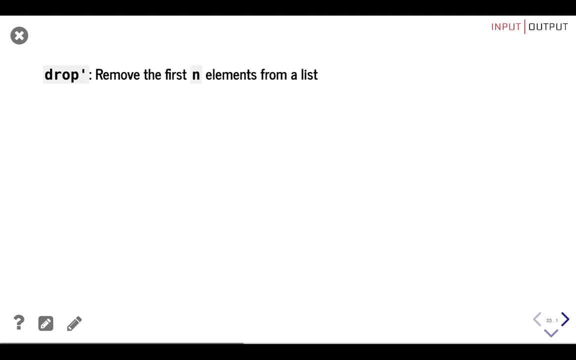 And because, in principle, we want to operate on the elements of the list, we can use a polymorphic type like this: Okay, this is new. We have two different arguments to take into account. now, The way to do this is to present all possible standard. 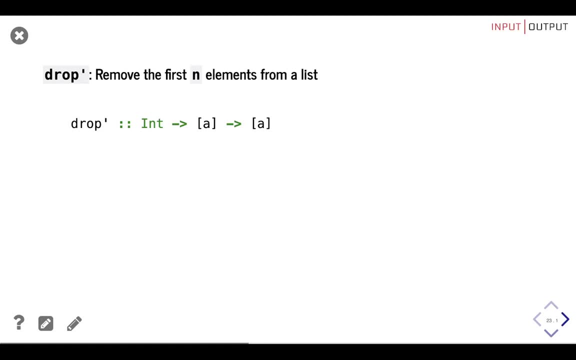 pattern combinations. Because we have numbers, we initially take into account the pattern for 0 and any other number, And because we have lists, we have to take into account the pattern for empty and non-empty lists. So we have four different cases, or the four different cases. 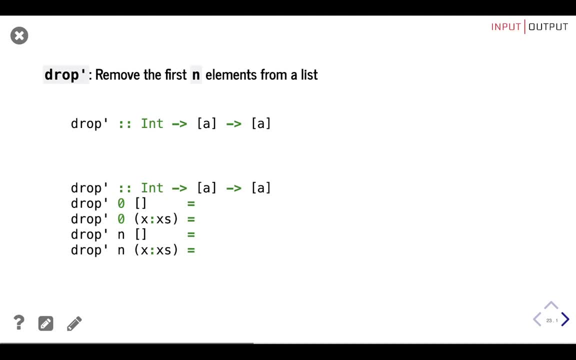 of possible combinations. As you can see, there are more things to take into account, but it isn't necessarily more difficult. Let's think about each case individually. In the first case, if we drop 0 elements from an empty list, it makes sense that the result will be an empty list. 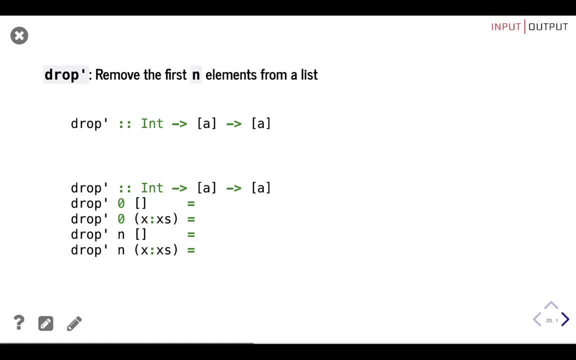 In the second case, if we drop 0 elements from a non-empty list, we return the same exact list. And in the third case, if we drop n elements from an empty list, we can return either an error or an empty list. 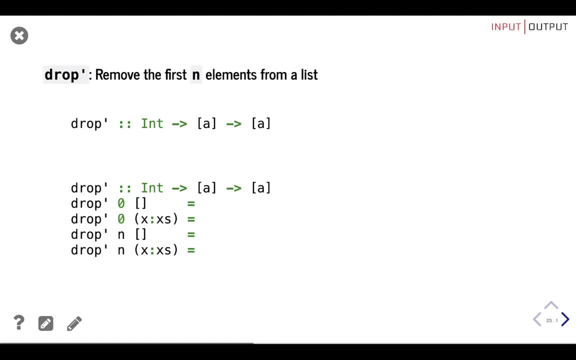 We choose to return an empty list. So, replacing those definitions, we get this. We completed three of the four cases. Now what about when we want to drop n numbers of elements from a non-empty list? We already have the first element separated from the list. 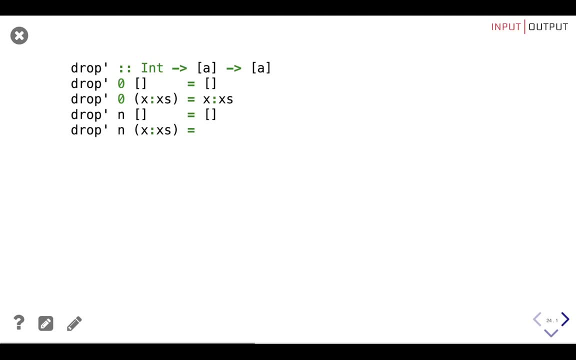 So if we remove that one, it's one less element to remove. But if we do something like drop n excess, the function will keep dropping elements until the list is empty. Luckily, there's an easy solution If we recursively call drop with excess. 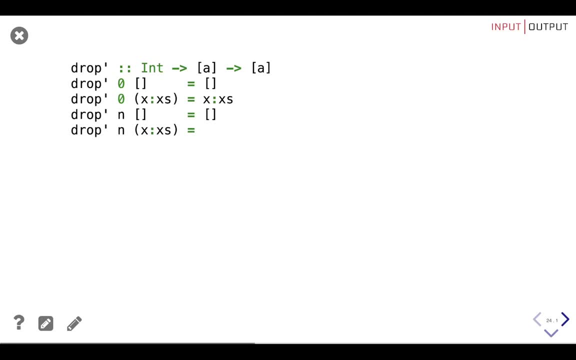 we'll be dropping one element on each recursive list, The first one, So we can subtract 1 from n on each call to keep it in sync. That way, if there are more than n elements, we will stop the recursion. when we reach n equals 0.. 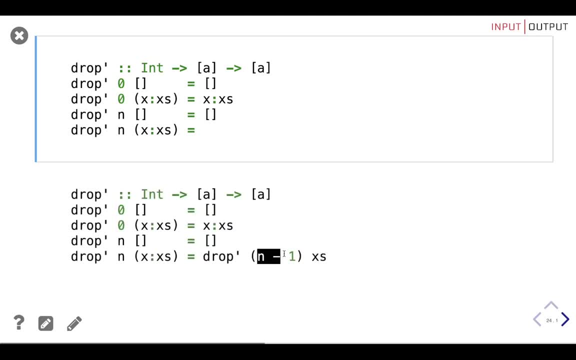 So we get this This way: both parameters are in sync. Okay, we have a working function, But there are a few things to remember. The first one is that both cases that take an empty list return an empty list, So we can ignore the int in those two cases. 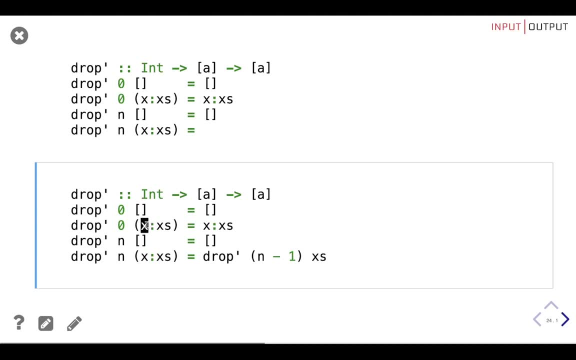 And also in the second case, we just pass through the inputs as the result, So there's no need to pattern matching. And finally, we don't use x in the recursive case, So we can ignore it Doing those changes. 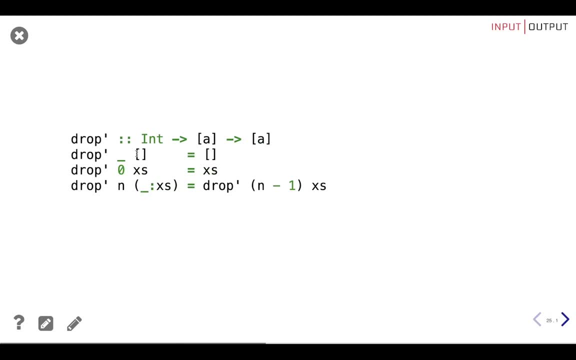 we get this For all the cases. when we have an empty list, we return an empty list. When we need to drop 0 elements, we just return the same list we got. And because we don't use n, we can just ignore it. 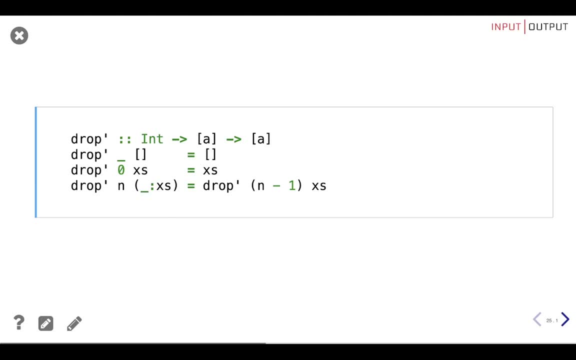 It looks like we arrived to our final drop definition, But did we really? What happens if n is less than 0?? Theoretically it doesn't make any sense. How will you drop minus 3 elements? But in practice, someone could be crazy enough to try it. 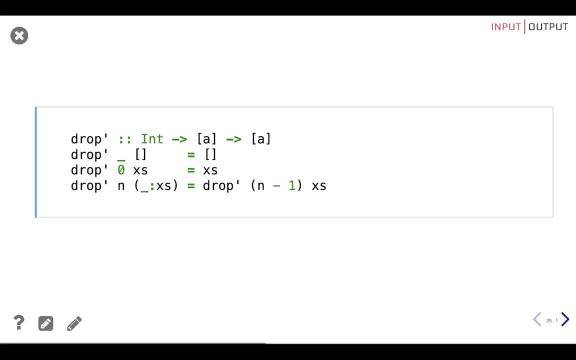 In that case our current function will keep dropping elements one by one until it runs out, because it will never get to the case of n equals 0. That could be a way to handle the case, But intuitively you would think that dropping a negative number of elements 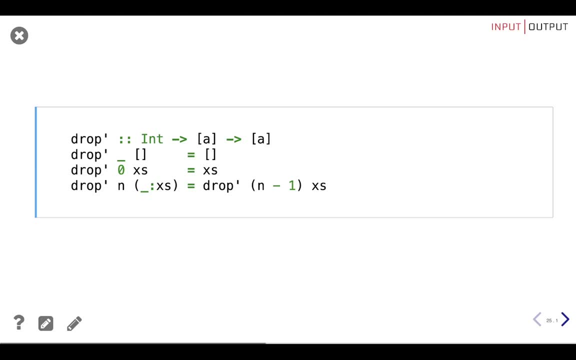 would do the same as dropping 0 elements meaning nothing. So we have to adjust our definition to accommodate that And to do it we can change the case that handles n equals 0 to handle n is less or equal to 0. 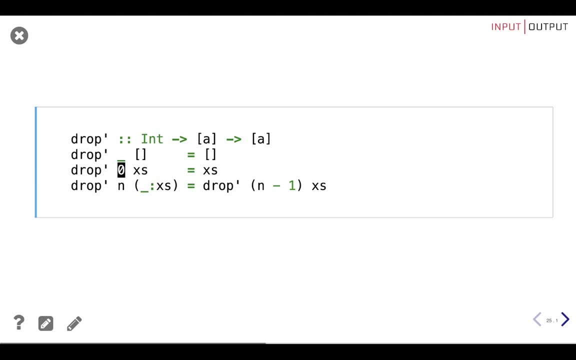 by binding the number to the variable n, like in this case, but in this case- and using guards to check for the desired property, like this. I want to remove all this. We don't need it so far, And in this case. 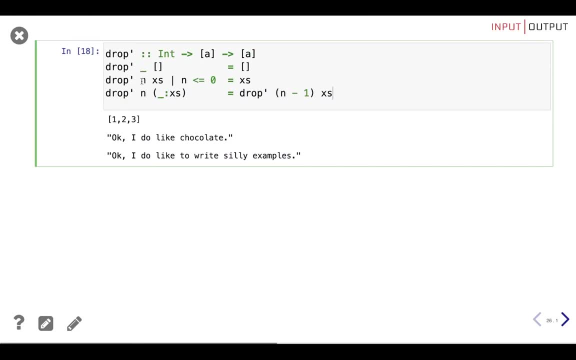 this is the only thing that it changes. Instead of pattern matching for 0,, we pattern match for any n and, using guards, we check that this n is less or equal to 0. In that case, and only that case, we take the initial list and return it back. 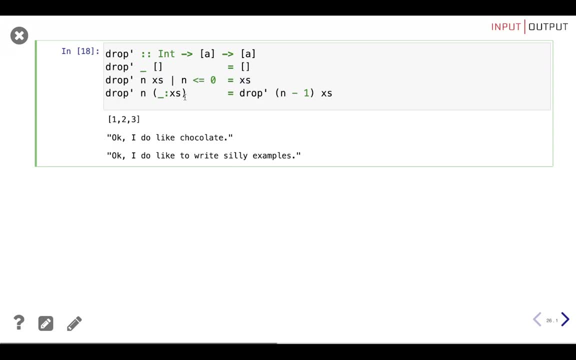 In any other case we fall back to the recursive case And to prove that it works here, we are dropping minus 3 elements from the list and we get the same exact list. And of course you can use the drop function and compose it with other functions. 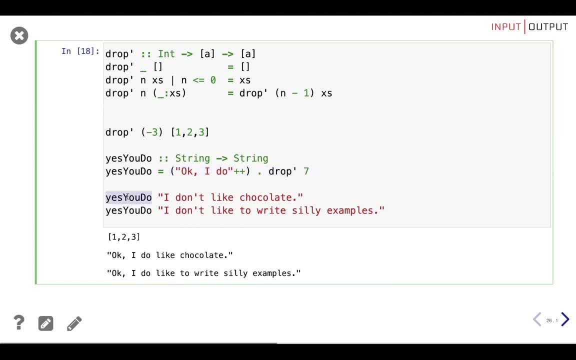 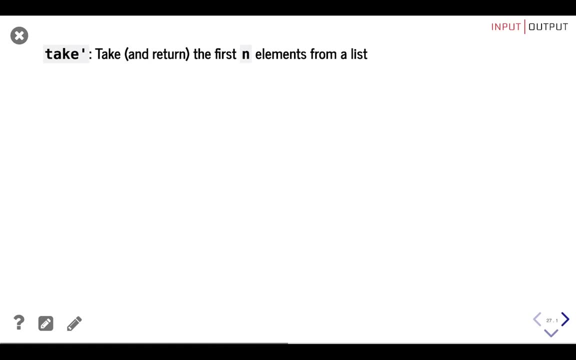 and also partially apply it to create incredible useful functions. Now let's talk about the take function. Take takes and returns the first n elements from a list. This function is oddly similar to the drop function: It takes an integer and a list and returns a list. 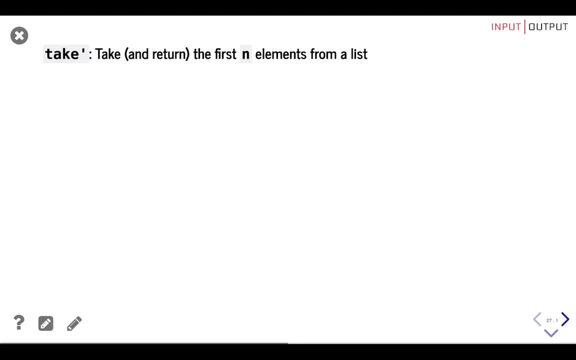 But this time the returned list contains all the elements from the first one up until n, Because we just saw a similar case. we'll do the first and second steps together. So we have a function that takes an int and a list and returns a list. 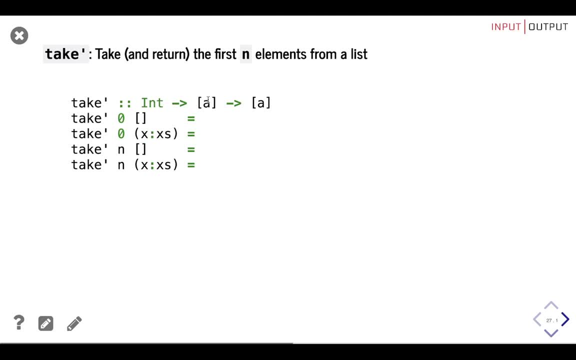 and we have all the cases for numbers and lists Same as before. let's think about each case individually. If we take 0 elements from an empty list, it makes sense that the result would be an empty list. If we take 0 elements from a non-empty list, 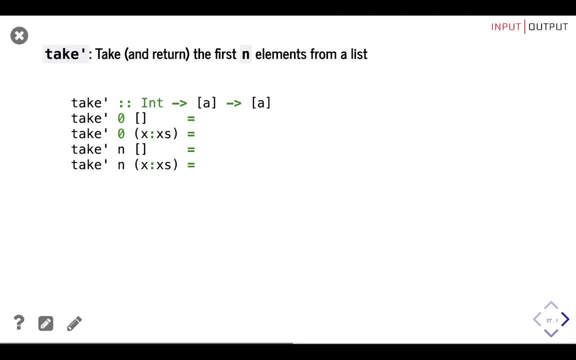 we take nothing, So we return an empty list. If we take n elements from an empty list, like before, we can choose to return an error or an empty list. We choose to return an empty list Replacing those three cases, we get this. 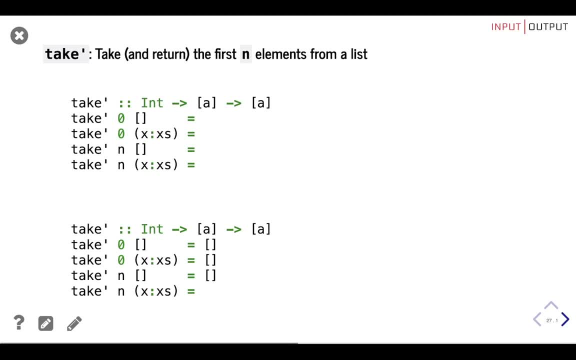 Well, that was easy. Now for the recursive case. Like the last time, we also need to reduce n by 1 on each step. But unlike last time, now we want to keep the element on each step, And there's an easy way to do it. 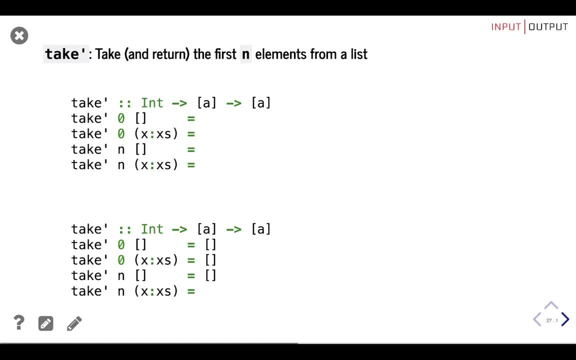 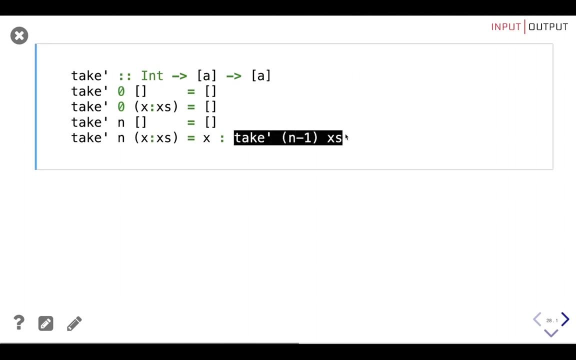 We can prepend the element using the const operator to a new list that will keep getting recursively bigger until we either reach n equals 0 or we run out of elements in the list. Translated to code is this Here: this part is the same one as drop. 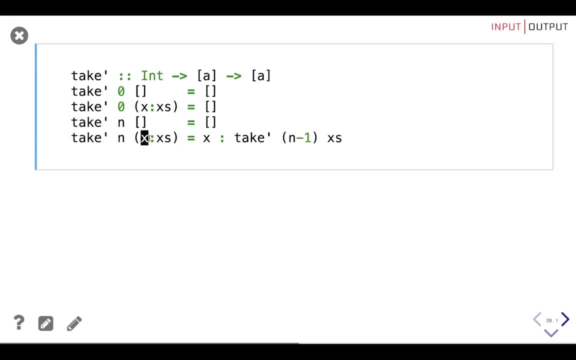 but now, instead of forgetting about the first number, in this case, we prefix it to the recursive call of take, So we will get a list at the end. Now we can simplify the expression in two different ways. If n equals 0, we don't care about the list. 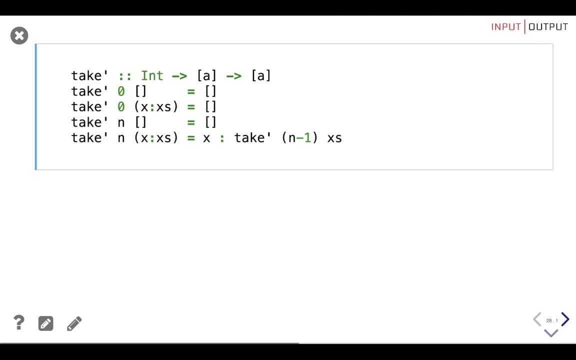 We will return an empty list anyway. And also, if the list is empty, we don't care about the number, We will return an empty list anyway. We can just do that and get this: If the number is 0, we ignore the list and return empty. 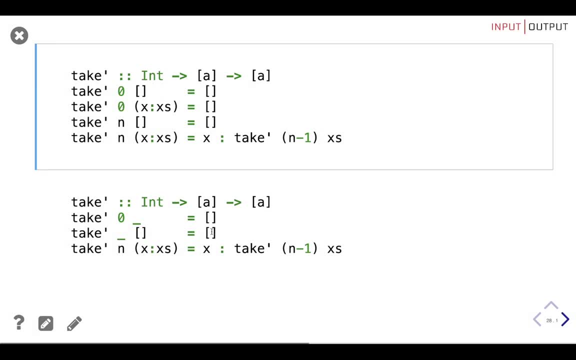 If the list is empty, we ignore the number and return empty list. We do have the same problem as we did with drop. Intuitively taking a negative number of elements should do the same as taking 0 elements. It should not return the whole list like now. 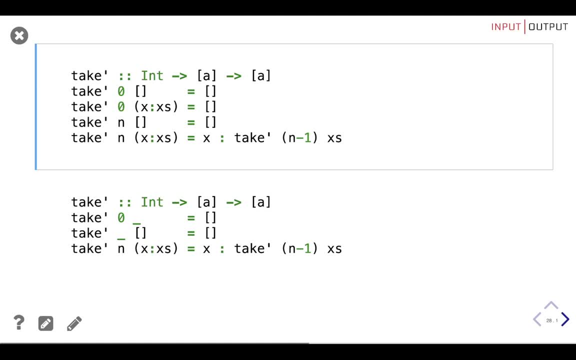 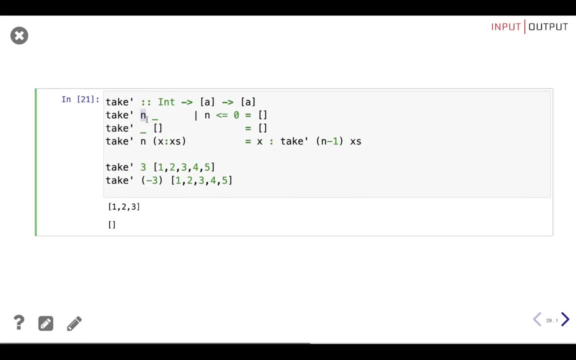 Luckily, we already know how to solve this problem. Same as with drop: We better match the value of n and we check in a guard that n is less or equal to 0. And that's it. We have our take function that works as expected. 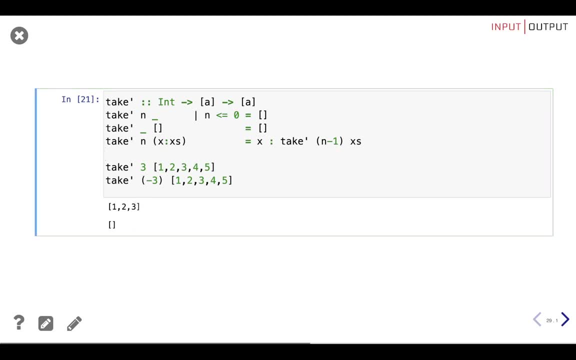 Now let's see how to define recursive functions. that takes functions as an argument. Let's start with the map function. Map is a higher-order function that applies a function to every element on a list. As always, let's start with the type. 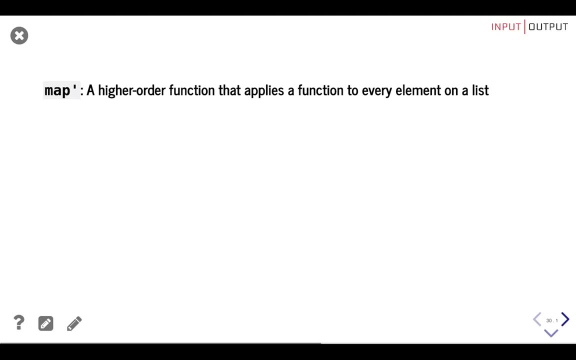 We will have a function and a list and we will return a list And, because we don't really know the function that will be passed as an argument, we will use a polymorphic type variable like this: The first argument is a function from A to B. 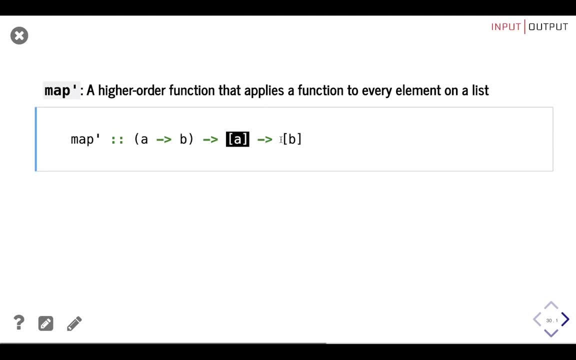 and the input list is a list of A's and returns a list of B's. Now let's enumerate the cases. In the case of a function, there's only one case. You get the function. So, taking into account the standard cases for lists, 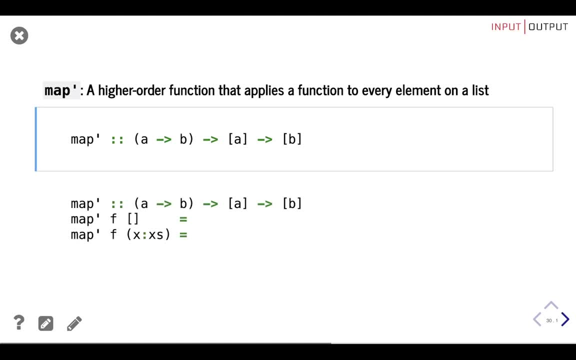 we get these two cases: The case for an empty list and the case for a non-empty list. If we don't have elements on the list, we just return the empty list, which will be our base case, And also we won't be using the function in this case. 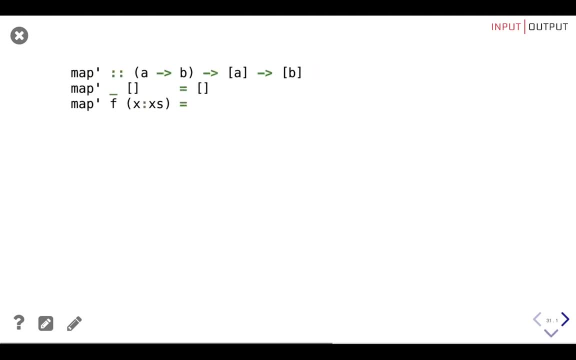 so we can just ignore it. Now for the recursive case. We have to apply the function f to every element and return the list. So we could apply f to the first element, x, and prepend it like before to the recursive call of using map applying to xs. 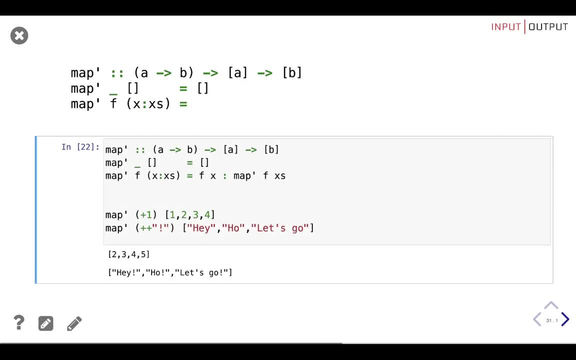 Like this And we got our final function. As you can see, we apply f to the first value and prepend to the recursive application of map to f and xs- the list without the first element. As you can see, we can pass the plus one function. 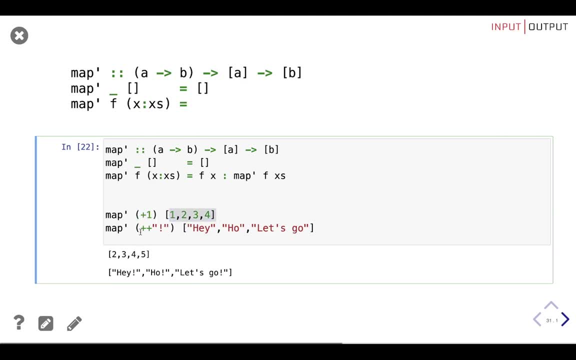 to add one to each element of the list. We can also pass the function to concatenate the exclamation operator to every word of the list, And we can do also more useful stuff, Because this is an incredible useful function And you will use it quite often. 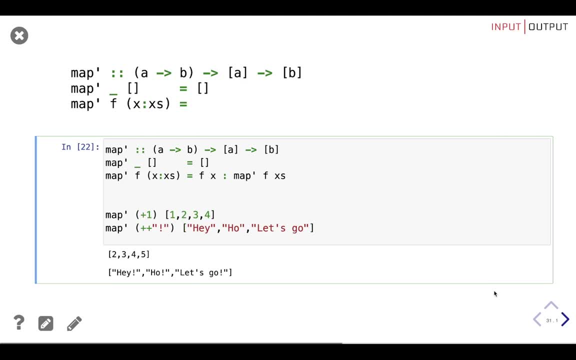 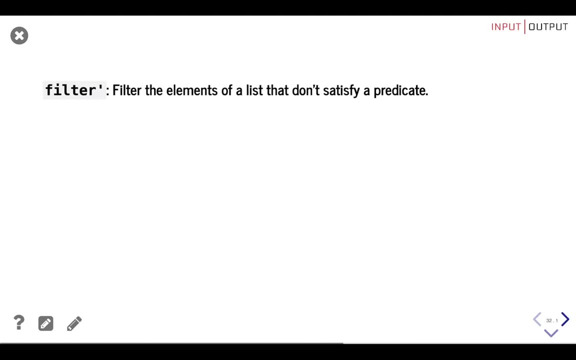 Now let's do one last recursive definition before learning about polls. Let's define the filter function. Filter filters the elements of a list That don't satisfy a predicate. We use this function quite a lot, So you know how it works. 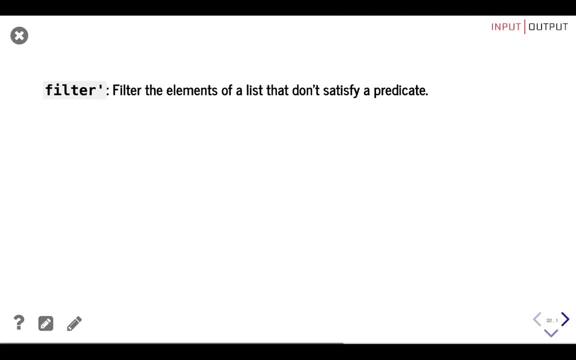 It takes a predicate and a list and returns a list with only the elements that satisfy that predicate. So translate it to the type We take a predicate, a function that returns a boolean, a list of a's and a list of a's. 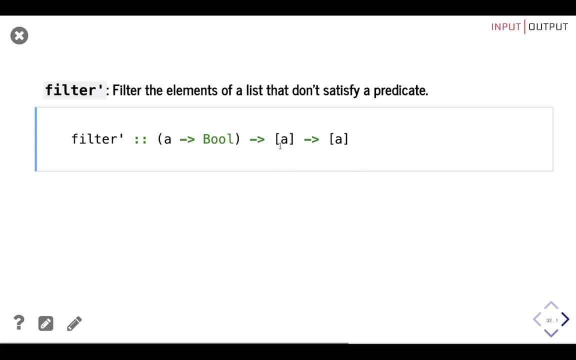 because we are not changing the values, We are just filtering and we will get an equal or shorter list as a result. Now, if we enumerate the cases, the first parameter is a function, So there's only one case, And the second is a list. 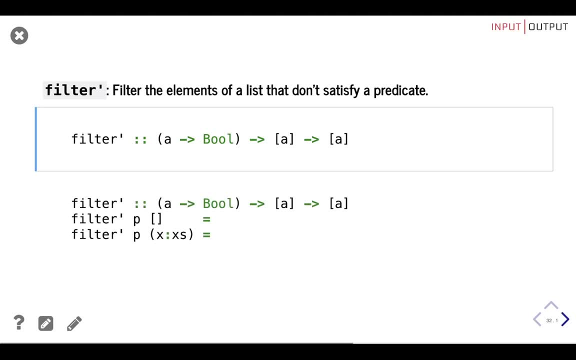 So it can be empty or a non-empty list, Because we don't have elements to be filtered. in the first case, we return an empty list And because we won't be using the predicate, we can ignore it. It is starting to feel easy, right. 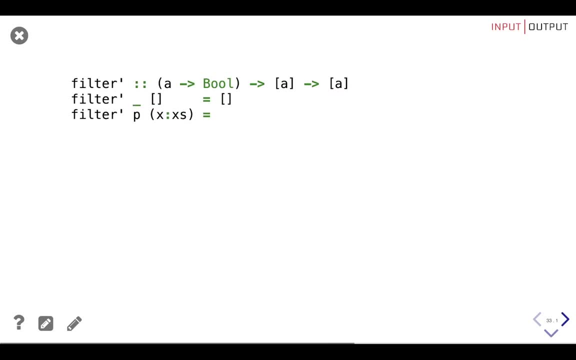 Now let's work through the recursive case. In this case, we have two situations. One is that the element does satisfy the predicate and the other that it doesn't. We could convey this in different ways: if-then-else expressions, for example: 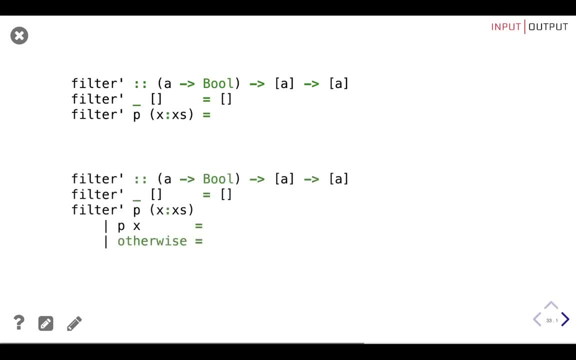 But I prefer using guards like this: If the predicate p applies to the first element, x returns true, we fault in this case, The case when we add the elements to the list that we will return at the end. Otherwise we don't. 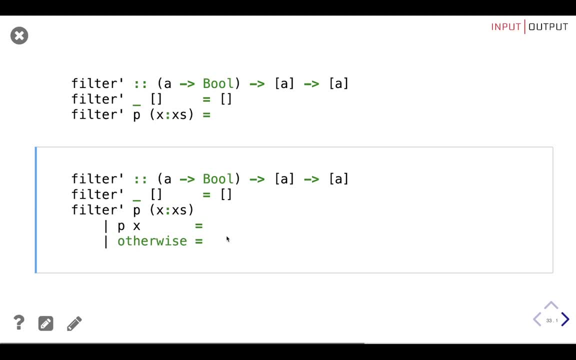 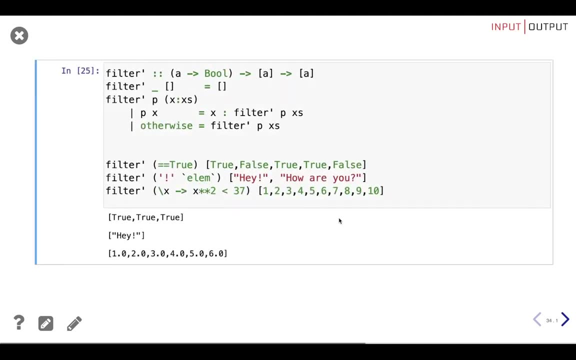 And in both cases we recursively apply filter to the rest of the elements of xs. Translating this to code, we get this. If applying the predicate to x returns true, we fall into this case. We prepend x and recursively apply filter. 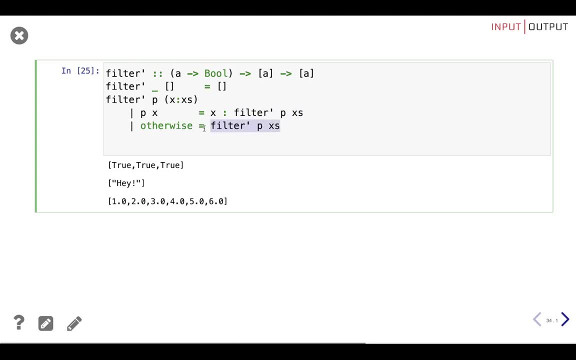 Otherwise, we recursively apply filter, but we don't prepend x, so it won't be in the final list. As you can see, there's a bunch of examples. We can filter all the elements that are equal to true, all the elements that contain the exclamation. 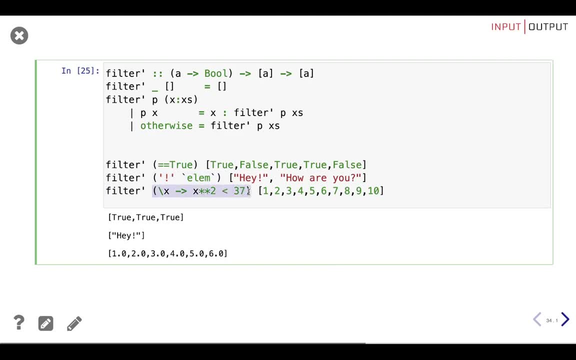 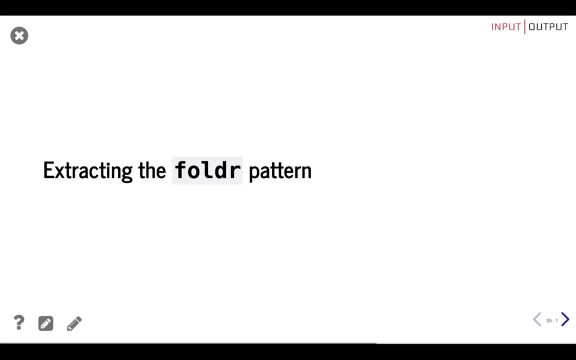 or we can filter all the elements that square are less than 37.. And that's it. You can filter away. We created enough recursive functions to start noticing some patterns. Let's talk about that. This is kind of an spoiler, but we are going to extract the fault pattern. 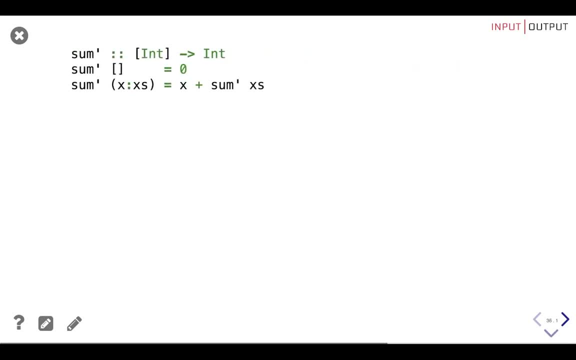 Now take a look at these previously defined functions. See if you can spot a pattern. We have the sum function function, the product function and the and function. As you can see, there is a pattern that repeats in every function. 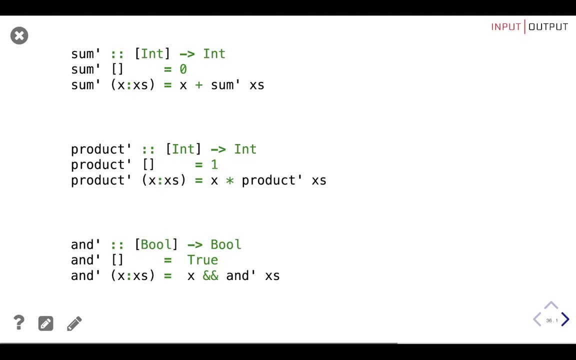 There is a base case for an empty list that returns a non-recursive value, and there is a recursive case for a non-empty list that takes the first value of the list and applies a function to combine it with a recursive call that processes the rest. 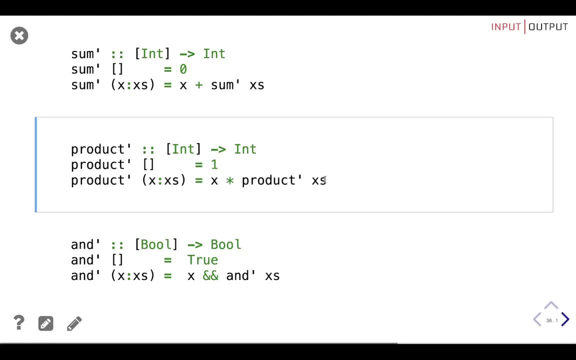 of the list. This pattern has a name. It's called primitive recursion. By now you know the drill. We are going to extract the pattern into its own function, But first notice that this pattern assumes that the function that combines the value 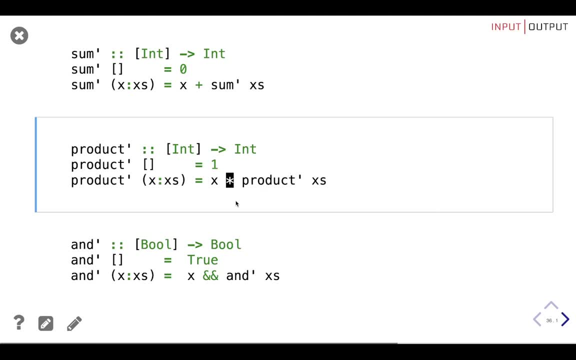 on the recursive case is an operator. To make it more general, let's modify them to use a prefix function before extracting the pattern. For example, the sum function will become this one. The only thing that we did is to change the function to a prefix function. 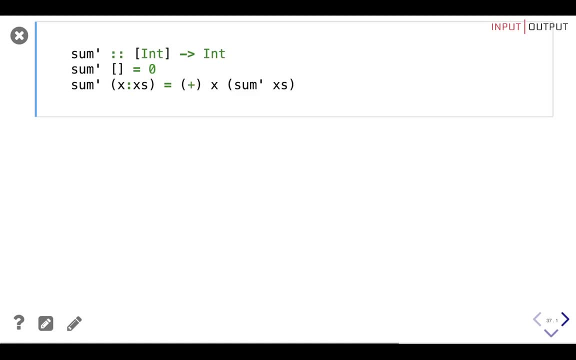 so it gets its two arguments to its right: the product function the same and the and function the same. And now we are ready to abstract the pattern. We are going to call the abstraction called r, because we are folding the list from the right. 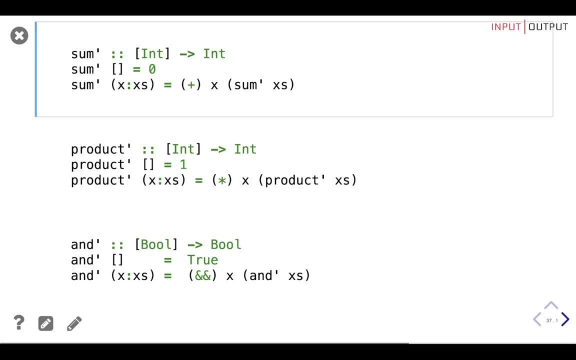 You will see what I mean when we use it. As always, first we start with the type. So we need three arguments. We need a function to combine the elements of the list, So it should take two elements. these two elements. 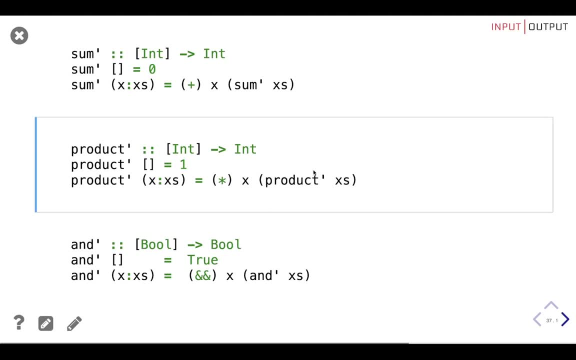 and generate a new one. We need a base value to start from and a list So we can write something like this: Notice that the elements inside the list can be anything, but not necessarily of the same type as the result. We don't know. 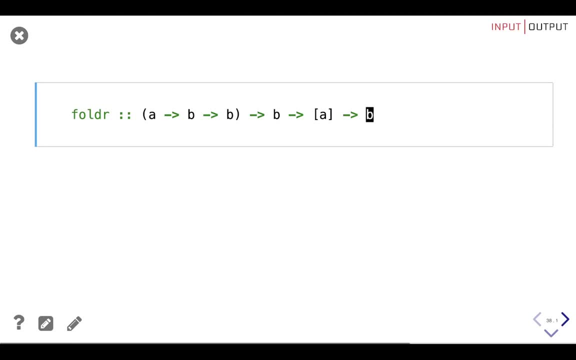 what the function will do. So we use a type a for elements on the list and a type b for the result, And for that follows that the base value has to be of type b, because it's the same type as the return value And the function. 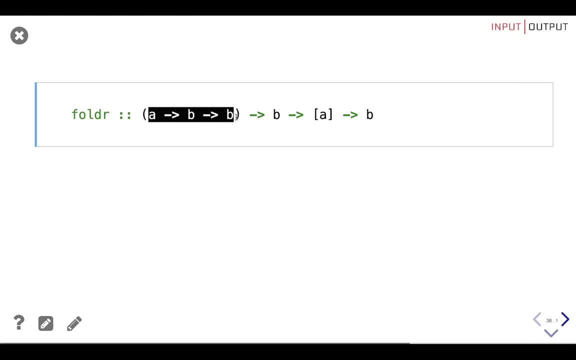 has to be of type a to b to b. Okay, now let's extract the pattern. Let's start by presenting the pattern and we'll go from there. Like we always do. we present the two cases. The case when the list is empty. 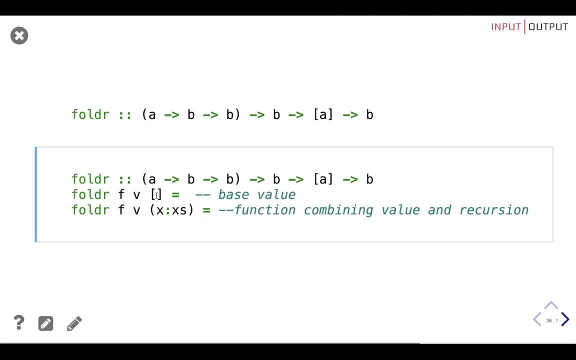 and the case when the list is not empty. When we have an empty list, like we said before, we have a base value and when we have a non-empty list, like we said before, we have a function- this function that will combine a value. 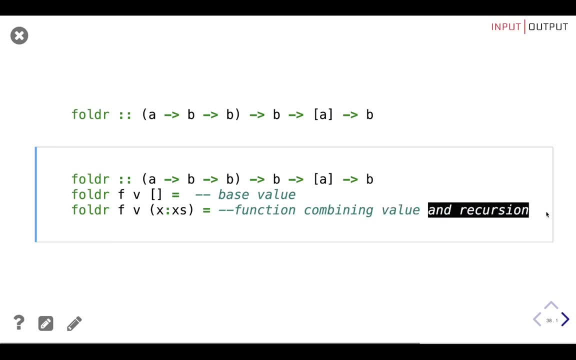 and a recursive call. We already have the base value- It's one of the arguments, And the recursive call is just applying the function f to x and recursively called fold r, but with xs instead of the original list. So we can do just that. 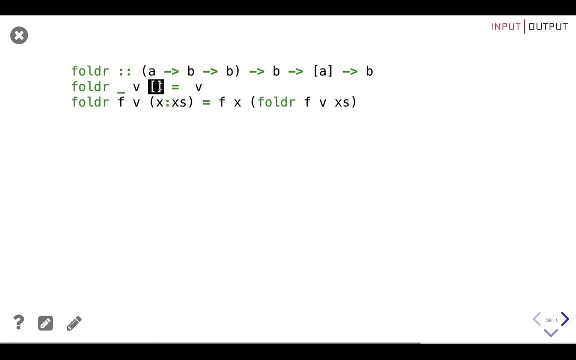 in the definition For the base value of empty list, we just take the base value and return it, And for the case for a non-empty list, we apply the function to the first value and as a second parameter we recursively apply the fold r function. 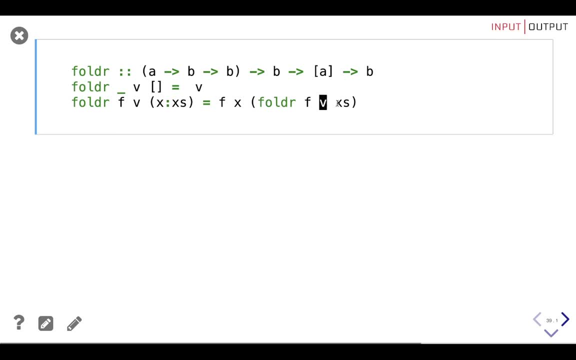 with the same function, the same base value, but just xs Done. We just extracted the primitive recursion pattern And to demonstrate that it's actually the same, we will pass the parameters needed to create the sum function and work through an example. 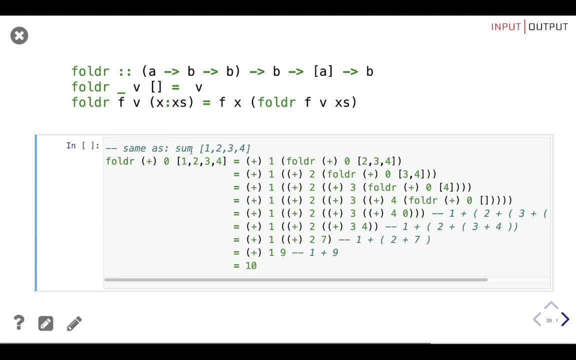 Let's see In this case to create the sum function and apply it to a list from 1 to 4, we can use fold r with the function that combines the values plus the base value of 0 and the list that we want to process. 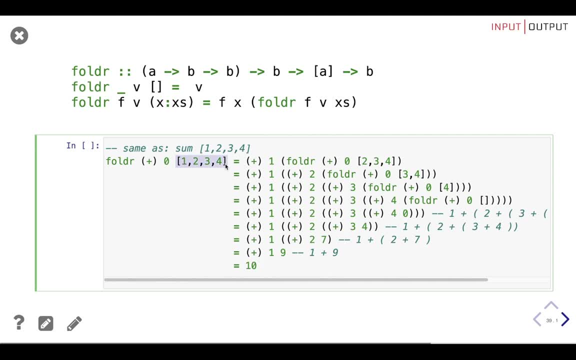 In the first call because the list is non-empty, we fold into this one. We write the function, the plus the first value, 1, and a recursive call for fold r with the same first two parameters but a shorter list. 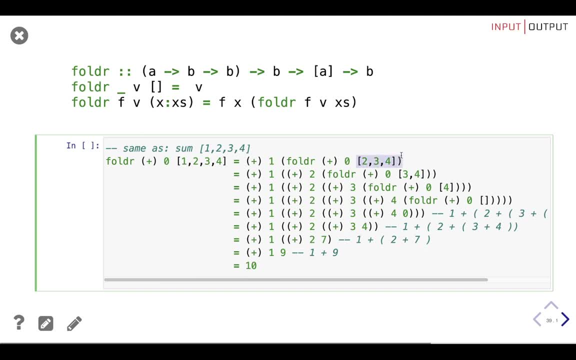 Because the list is still not empty. we'll do the same here, because the list is still not empty, et cetera, et cetera, up until here. Here the list is empty, so we fall into the first case. 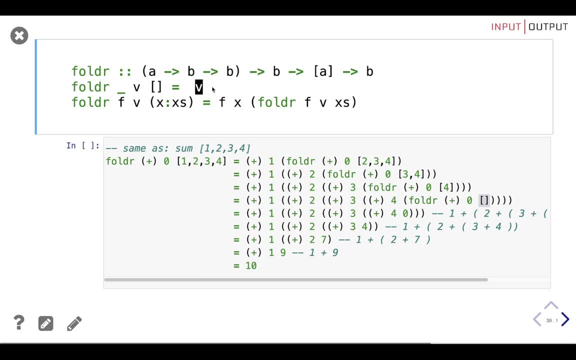 when we just return the b And the value in this case will pass as 0, so we return 0. And we get this expression Kind of hard to read. but in this case we have the function. we have the function plus. 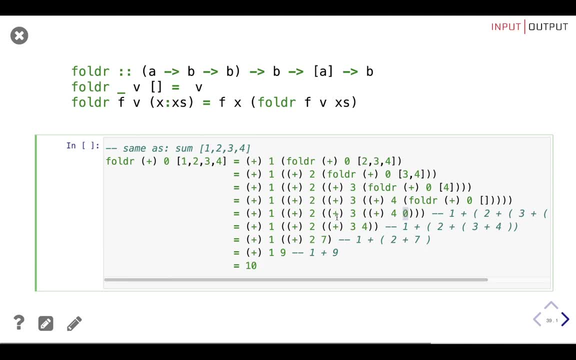 applied to 4 and 0. And then we have the function plus applied to 3 and the result of applying the function plus to 4 to 0. And so on and so forth. To simplify it, I will convert it back to an infix function. 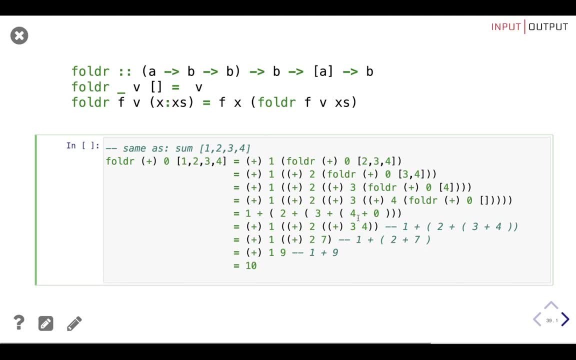 and we get this. As you can see, we start applying the function from the right of the list to the left of the list. We start with the final number and work through the initial number. That's why it's called for right, because we fold it from the right. 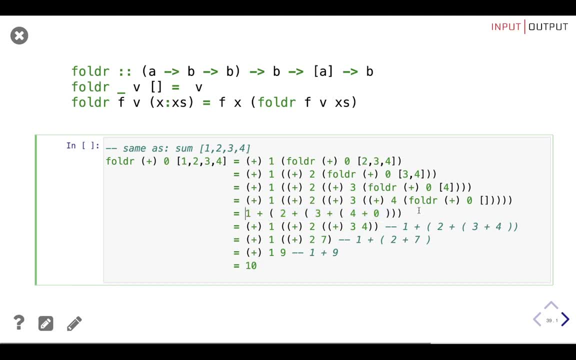 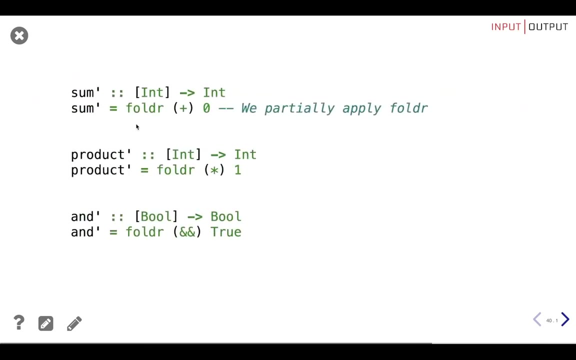 to the left, And if we simplify the expression, we end up having 10.. Now we can replace it in our previous definitions to get a much clearer and concise code. like this, We partially apply foldR with the function and the base value. 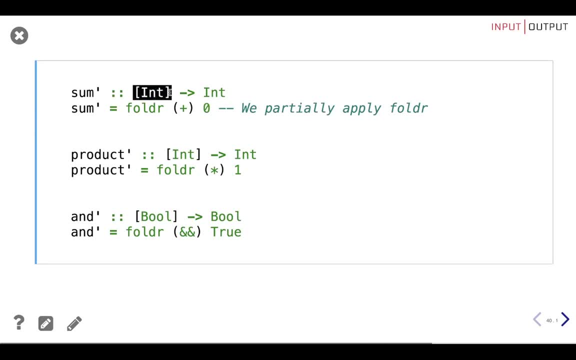 so we can get the sum function. that takes the list to be reduced. The product function is the same, but we pass the product operator and the initial value of 1 and the and function the same with the and operator and the base value. true. 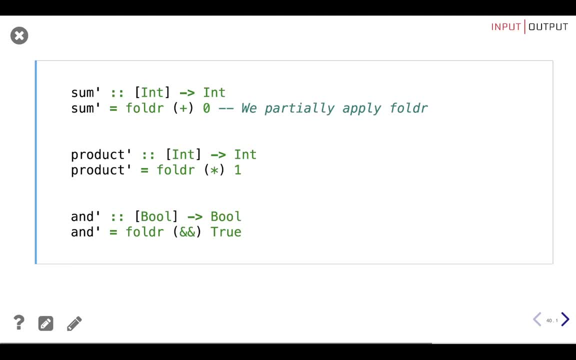 If, while defining a recursive function, you find out that you are using this pattern, use foldR instead. That way, everyone, including you two months later, will instantly understand what the function does, without needing to figure out the recursion. Remember that foldR. 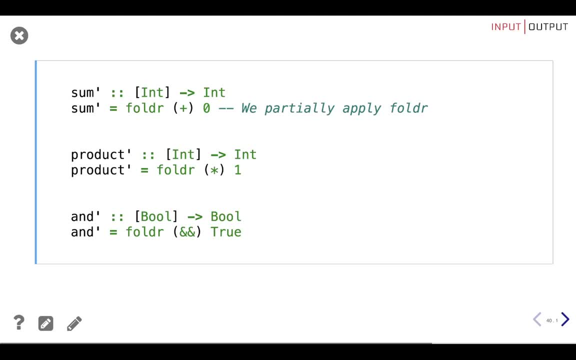 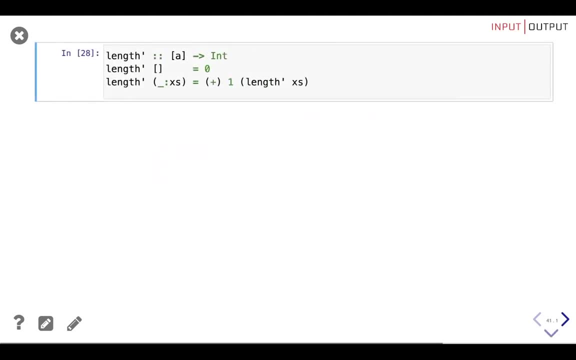 comes already in Haskell Speaking, of which the length function fits almost perfectly in the pattern. The only difference is that we ignore x and add a constant value instead. If we could just hard-code the first parameter of the plus operator, that would be perfect. 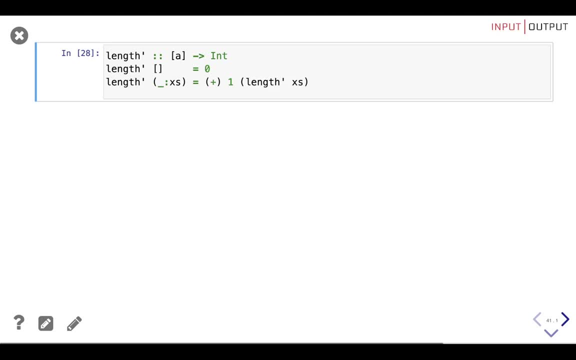 Well, why don't create a function that does just that and pass that function instead of plus? We just need to take two parameters, ignore the first one and add one to the second parameter. We can easily do that with a quick lambda function. 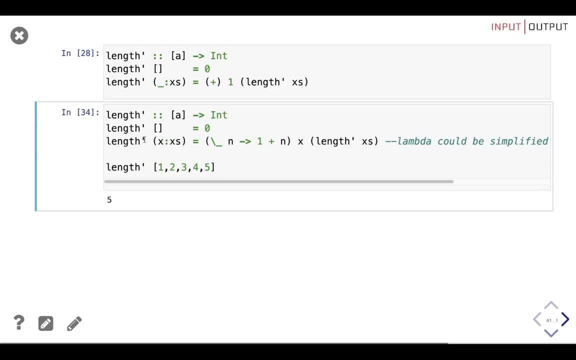 Here length is defined almost exactly the same as the sum function, but instead of using the plus operator we use this lambda function that ignores the first argument and just adds one to the second argument. As you can see, it works like a charm. 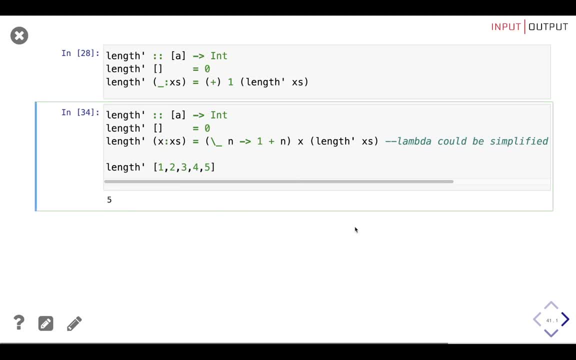 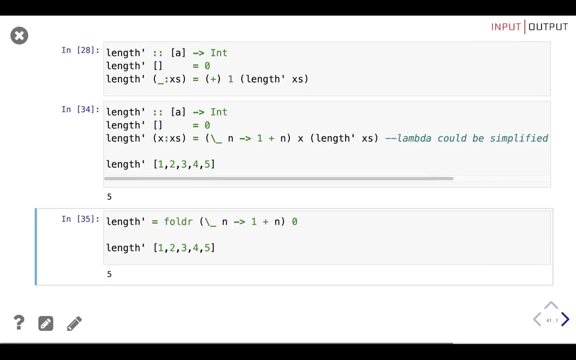 And boom. Just like. that length perfectly fits the pattern, So we can replace it with fault r. As you can see, there's certain flexibility. For example, we could implement reverse with fault r like this: Here we are using a lambda function. 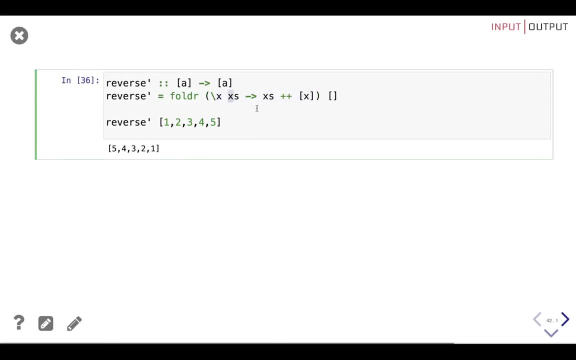 that takes the first and the second parameter, flips them and concatenates them. So it seems like we could use fault r all day long. But it's not all roses If, for example, we use reverse with a thousand. 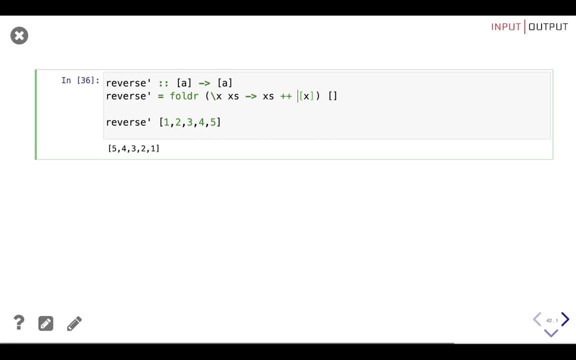 or ten thousand or even more numbers. the toll of using the concatenator operator grows bigger and bigger, Why? Well, let's see how the concatenator operator is defined in the base library. As you can see, in the recursive case, when the concatenator operator 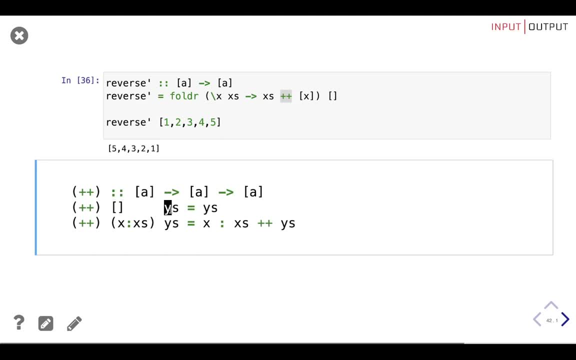 has an empty list as a first argument and any list as a second argument, it returns the second list because the first one is empty, But if the first list is not empty, it takes the first value and prefixes it to the recursive call. 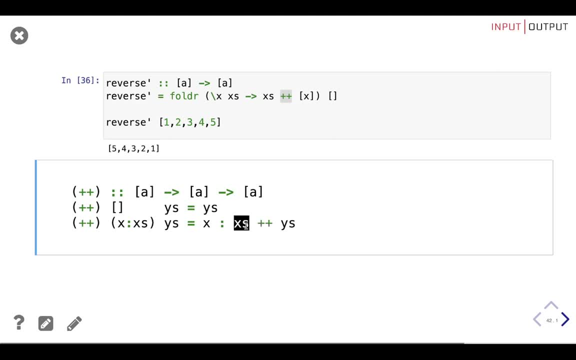 of concatenating the rest of the first list and the second list. As you can see in the recursive case, each time we want to add two lists, we first need to work through all the elements of the first list and then we add the second list. 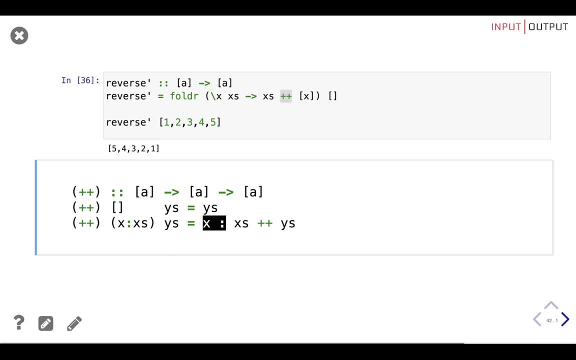 at the end. So if we have a list ten times bigger, we have to wait ten times more for it to complete, meaning that it takes a linear time in the number of elements of the list to finish. What does that mean to us? 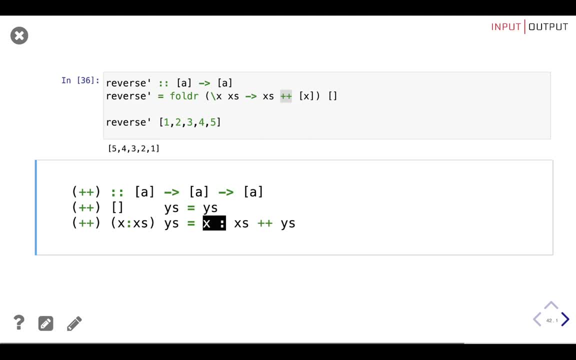 It means that on reverse recursive call, each time we want to move an element from the front to the back of the list. meaning every time we do a recursive call we have to work through the entire list every time If the list is long enough. 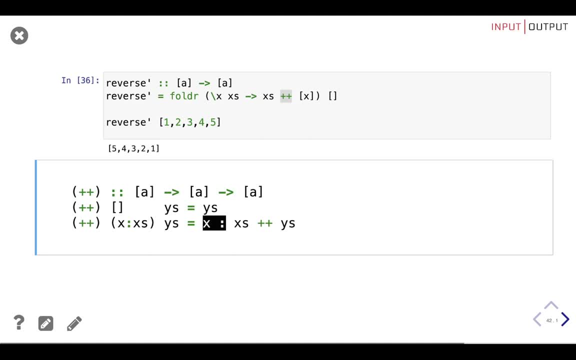 you could go for a run while waiting for it to be reversed. But don't worry, I wouldn't leave you hanging like that. There's a neat solution for this: If we could work through the list from left to right instead of from right. 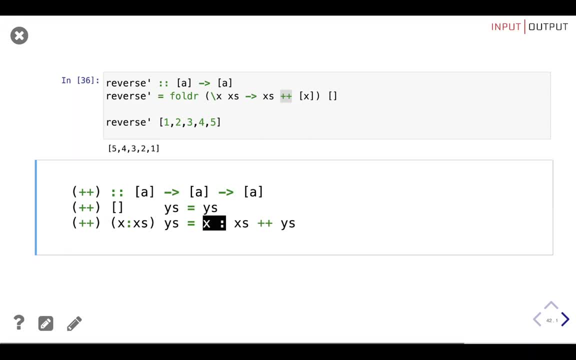 to left. we could use the cons operator instead of the concatenator operator And in each recursive call we will add the element at the very beginning, not walking through the entire list. as needed, Enter the foldL function. FoldL does the same. 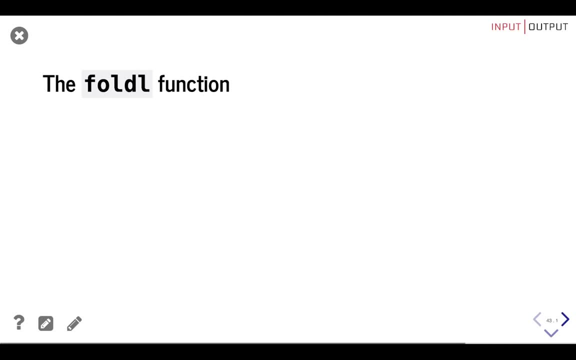 as foldR, but traverses the list from left to right. These are both the definitions. As you can see, the difference lies in the recursive case. In the foldR case, we apply the function to the first element and then the second parameter. 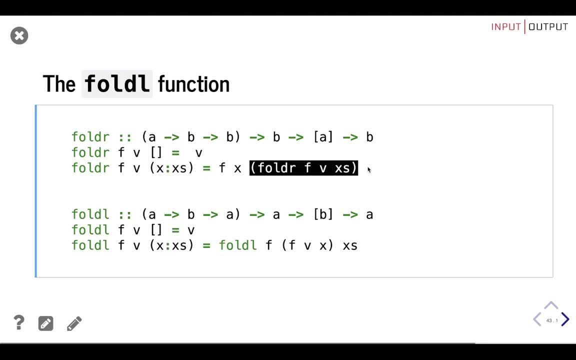 is the recursive call of foldR, But in foldL the recursive call is at the very beginning, with the same function but with the modified second parameter and modified list. This second parameter is usually called the accumulator because it accumulates the changes. 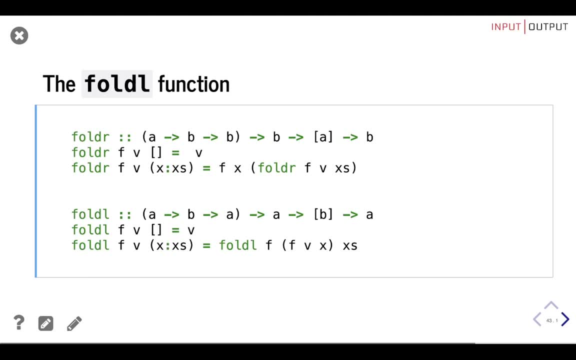 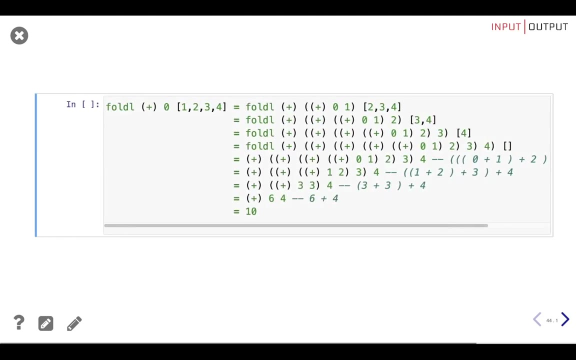 It's a little harder to see because we didn't extract it from a bunch of examples. But to account for that, let's see what happens step by step. when we replace foldR with foldL in the sum function, We applied foldL to the plus operator. 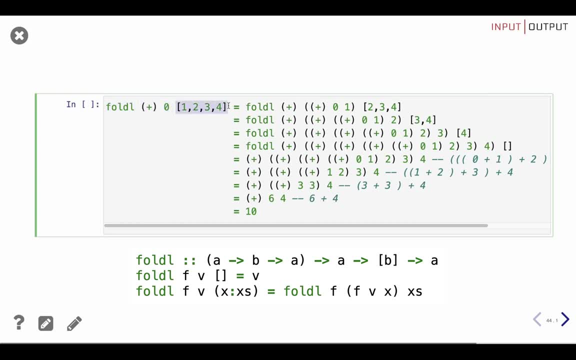 zero as the base case and the list one through four same as before. In this case, because the list is non-empty, we apply foldL again. The function is the same, but here in the accumulator we have the result of applying the function. 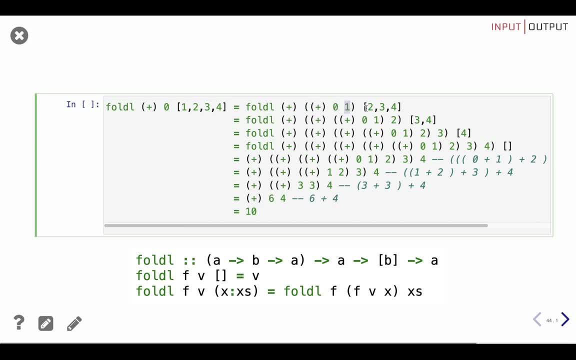 to the base value and the first value And as a third parameter we have the reduced list. Because the list is still not empty, we do another recursive call on foldL when we again the first parameter is the same: the plus function. 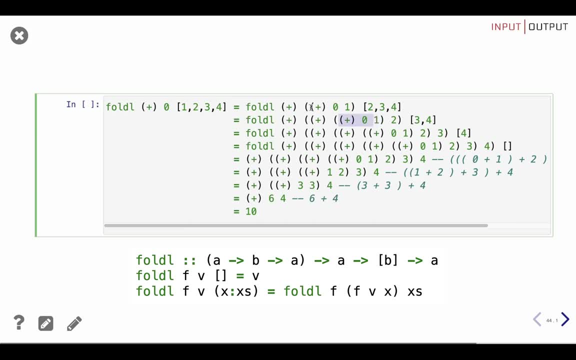 but the second parameter is the same value as before, but added to the second value And of course the list is one element shorter. We keep accumulating the changes in the second parameter and reducing the list in the third parameter up until we get an empty list. 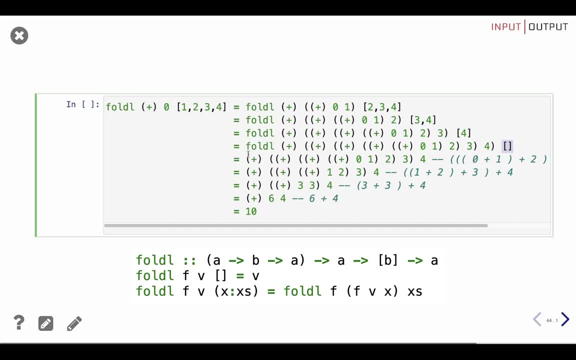 In that case we stop the recursion and we get this final expression: We add zero plus one, and then we add this with two, and then we add the result of this with three, and so on so forth, changing the function to become an infix function like: 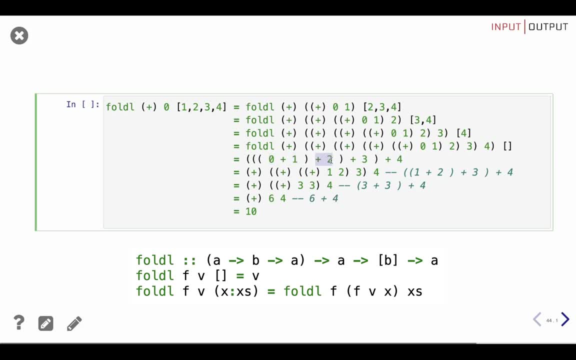 we did before. We get this zero plus one and the result of that plus two, and the result of that plus three and plus four And we get the same result. But now we can use the cons operator to join the values instead of the concatenator. 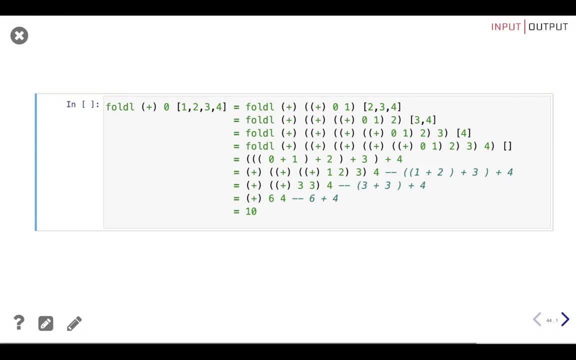 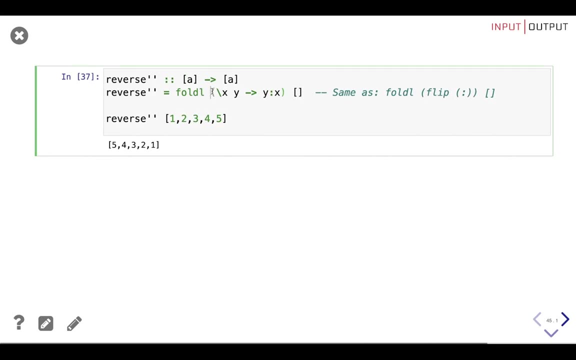 operator. Taking that into account, we can do this. Instead of using fold R, we use fold L, and now the result is this: Now we can combine them using the cons operator and we get the same result. Now we can compare the speed of the. 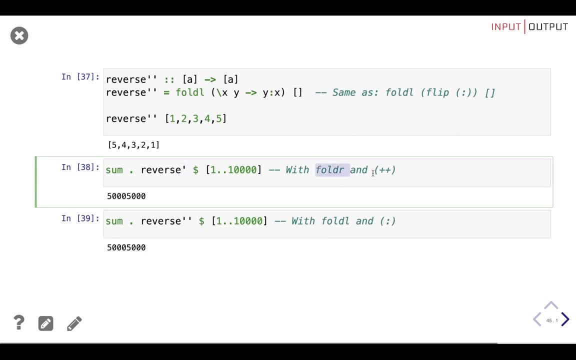 two functions by reversing a list, for example from fold L and the cons operator, And I sum the results so you don't get a long list of elements. If you run these two cells separately, you'll see the difference And also you'll see even. 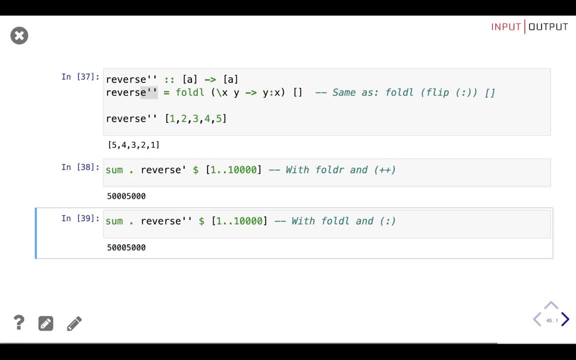 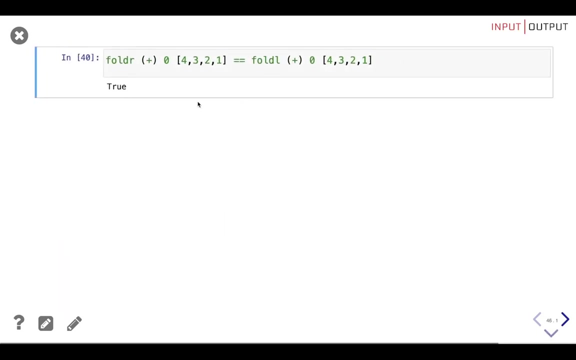 more than fold R, For example, the operator itself matters. So far we haven't encountered this because, for example, in the addition operator, if we use either fold R or fold L, we get the exact same result. But let's consider the minus operator, The result. 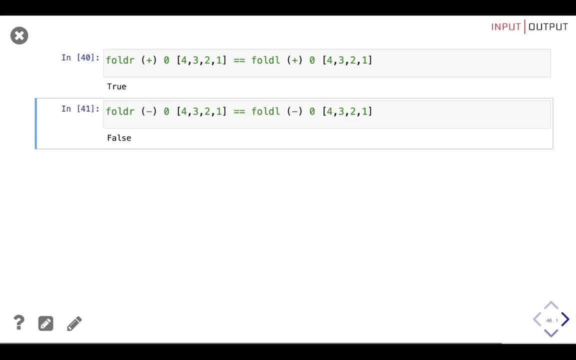 is not the same if you go from left to right than if you go from right to left. This is false, because if we write fold R, we get the same result as if we write fold R. we get the same result as if we write fold R. 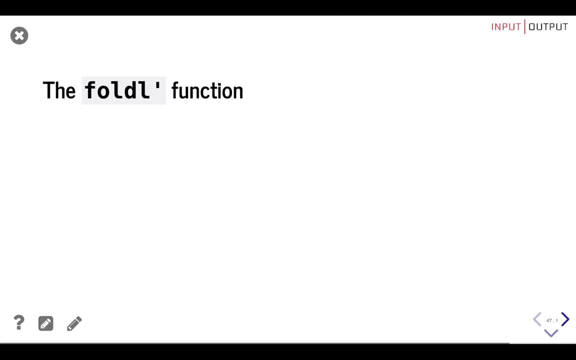 we get the same result as if we write fold L. In both fold R and fold L cases we saw that we keep stacking up expressions until the end And then we reduce them. We see that we can't do much for fold R, since we don't 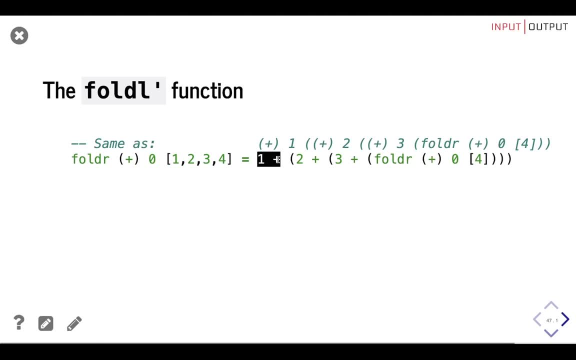 have a single operator with both arguments, For example one plus, and we need to reduce these expressions, and for this we need the recursive function first. But if we take a look at the same intermediate step, but in fold L, we see that we could totally reduce. 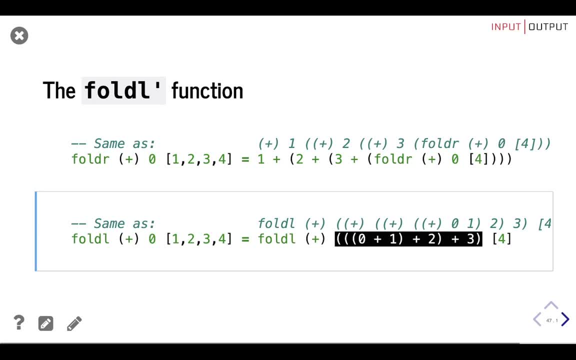 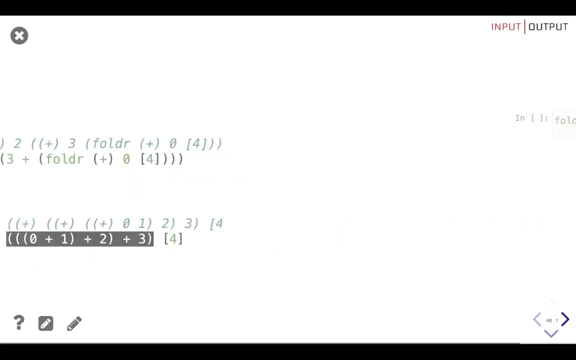 this whole expression to 6 before continuing with the same exact result. The difference is that fold L prime reduces the expressions at the intermediate steps, So it's more efficient because it doesn't build a huge thump. So if we use fold L prime, 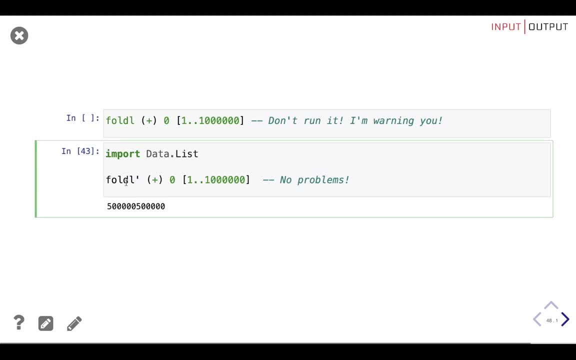 we could reduce the expression of fold L prime. Another detail is that fold L prime does not come with the base library in Haskell, So this raises a question: When should you use each fold? Usually, the choice is between fold R and fold L prime. 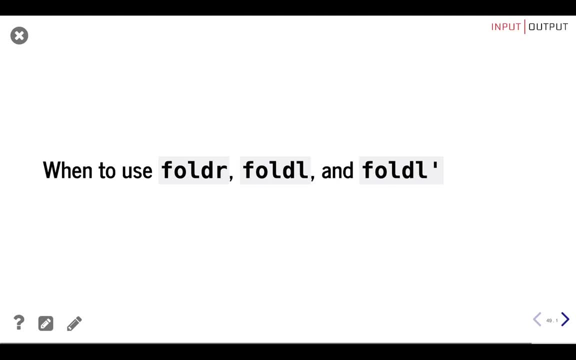 Fold L and fold L prime are the same as fold L prime. However, that's not the whole story. I'm going to give you some rules of thumb, from least to most used fold. When should you use fold L? When to use fold? 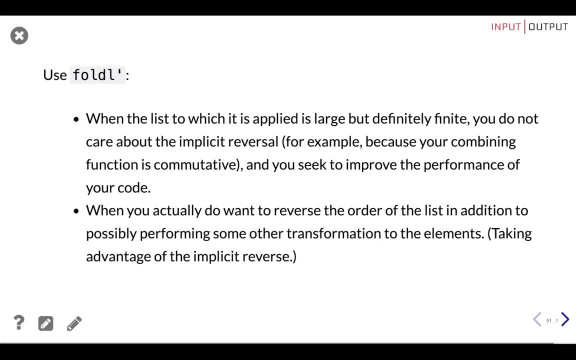 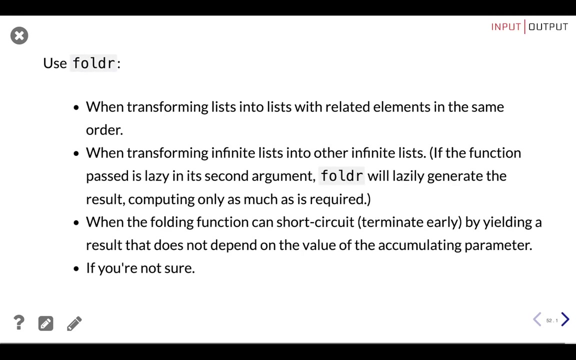 L prime When the list to which is applied is large but definitely finite. You don't know care about the implicit reversal, For example. your function is lazy in its second argument. fold R will lazily generate the results in the same order.